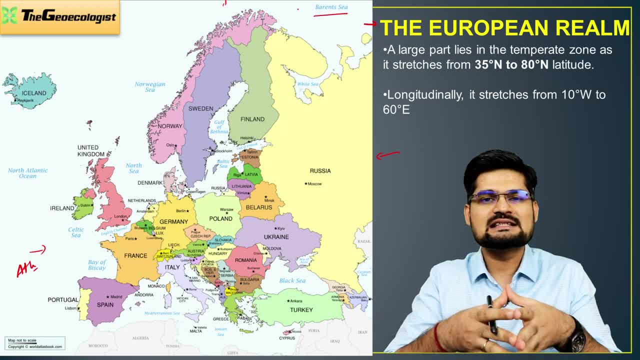 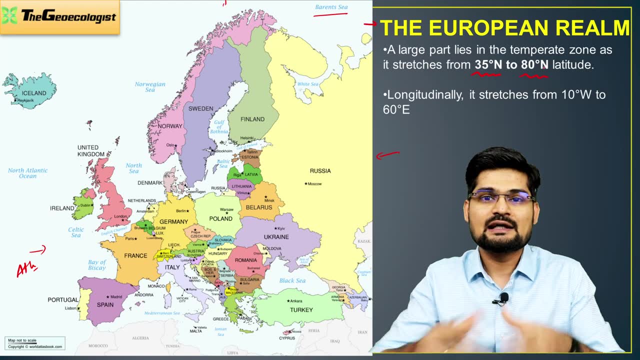 Atlantic Ocean Towards the Barents Sea. if you observe, this is the stretch and if you observe carefully, 35 degree north to 80 degree north is roughly the latitudinal extent. It means this entire landmass lies in the temperate belt to polar belt or sub polar belt and then longitudinally 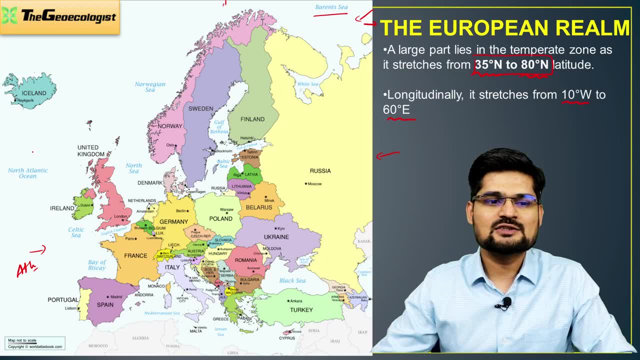 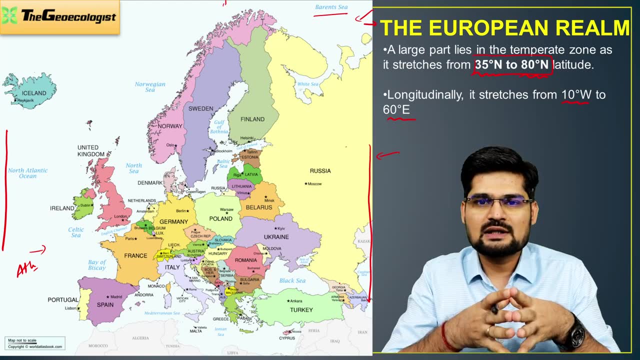 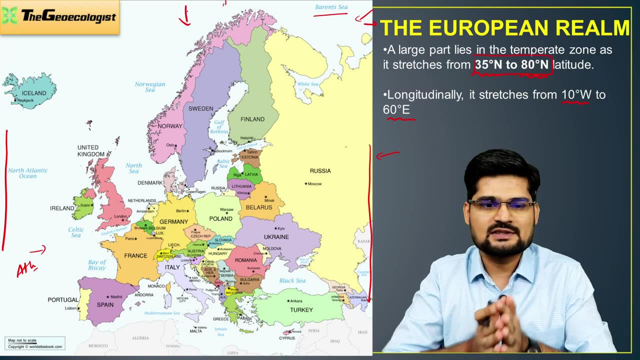 if you observe 10 degree west to 60 degree east, So this is the longitudinal profile, if you observe carefully. So this is the extent covering this particular landmass that we say is European realm. If you observe in European realm, these major countries can be observed on the map itself. 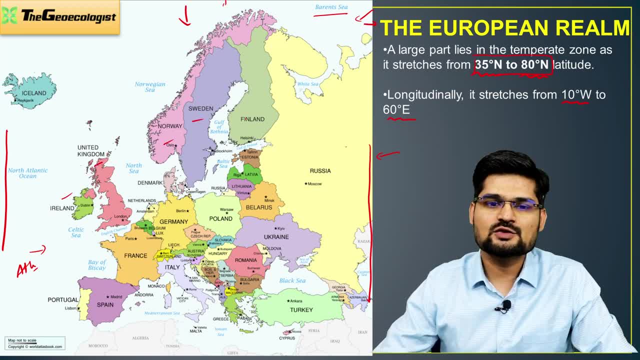 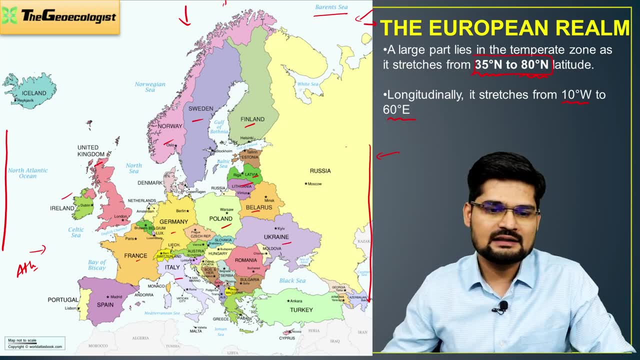 So if you observe United Kingdom, Ireland, then you have Norway, Sweden, Finland, then Belarus, Ukraine, Poland, Lithuania, Latvia, Germany, France, then you have Italy, Spain, Portugal, so many countries that you observe carefully here and I'm sure you must have. 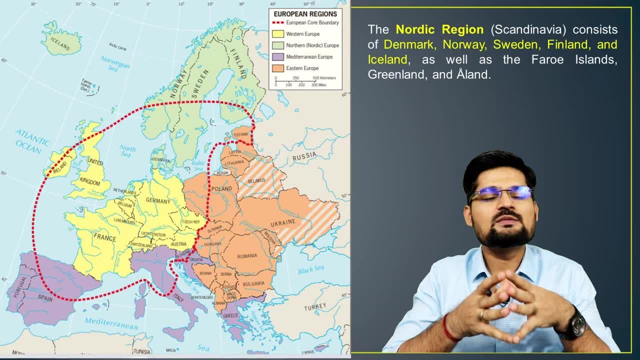 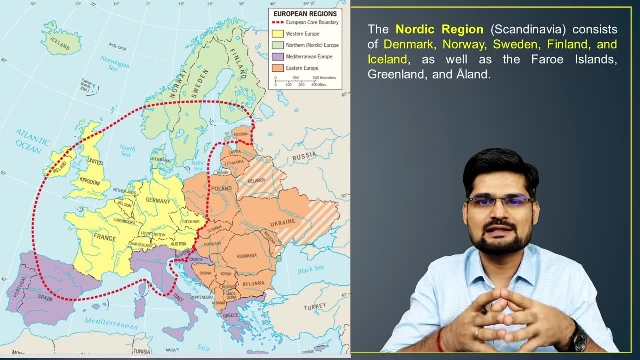 looked into these countries earlier as well. So now let's observe the regional classification of Europe and divide the Europe into several sub regions Which can be used for these studies. So first, if you observe, is this yellow color on your screen which is representing the 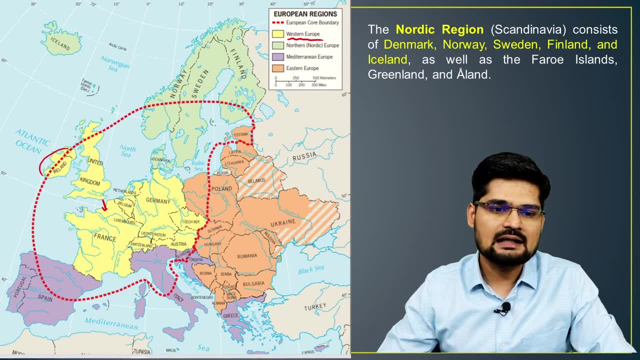 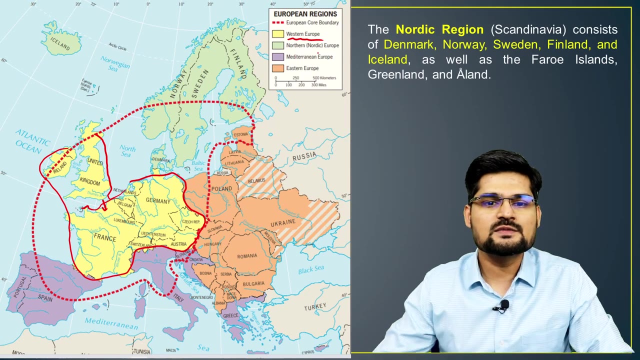 Western Europe, right? So this entire Ireland to the stretch of France, Switzerland, Austria, Czech Republic. then you have Germany, Netherlands, Belgium, United Kingdom, France, Luxembourg. all these areas are part of Western Europe as a region. Then, if you observe the northern region, which is Nordic Europe and also known by the name: 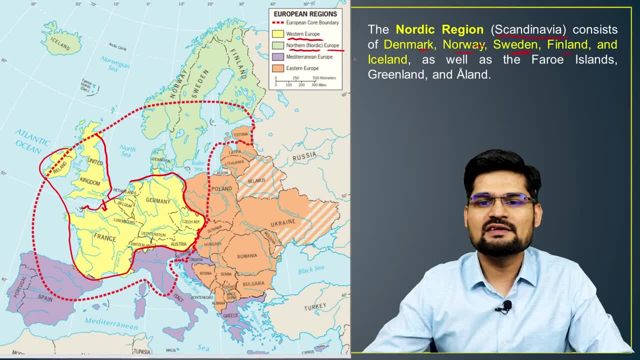 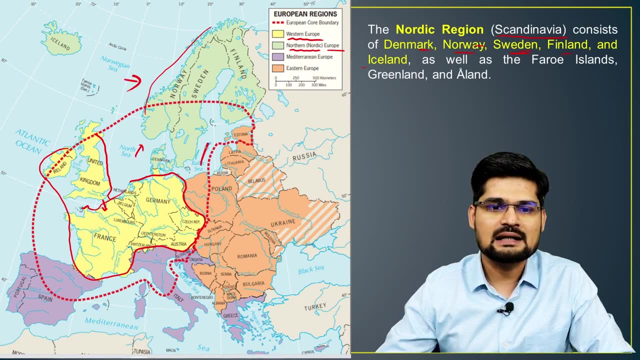 Scandinavian countries Like Denmark, Norway, Sweden, Finland, Iceland. So if you observe these areas near Norway and sea here, and also if you observe the North Sea out here, Baltic Sea out here. So these states which are also sometimes referred to as Scandinavian countries. 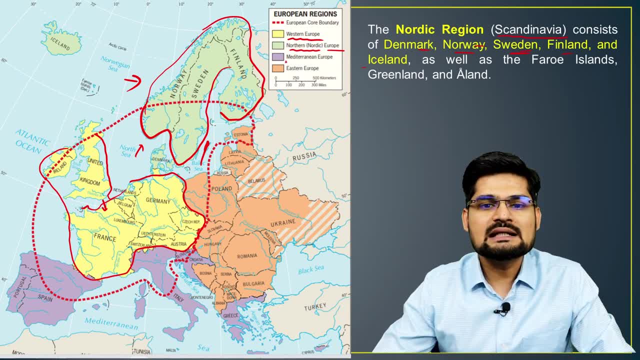 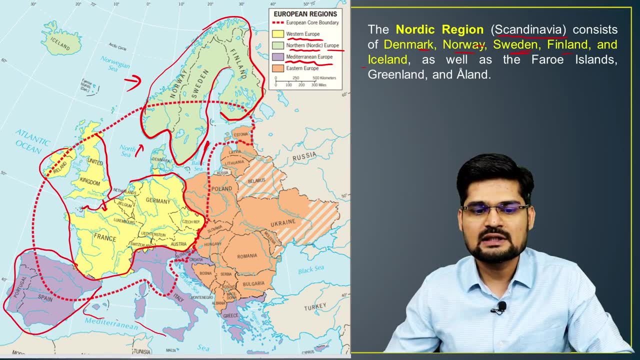 These are the northern region of Europe. Now come to the Mediterranean Europe, And obviously it's near the Mediterranean region. So Portugal, Spain, then you have different islands in the Mediterranean region, Then further you have Italy, Greece and Croatia And Croatia, Slovenia and others. 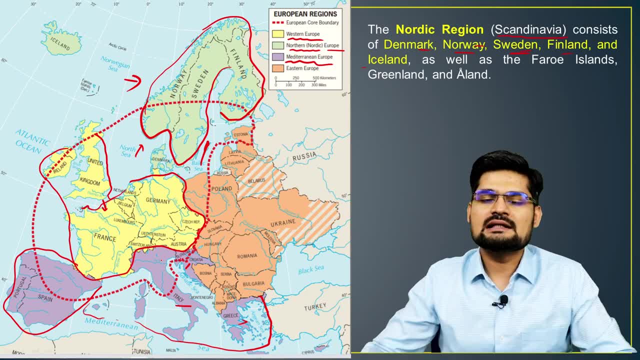 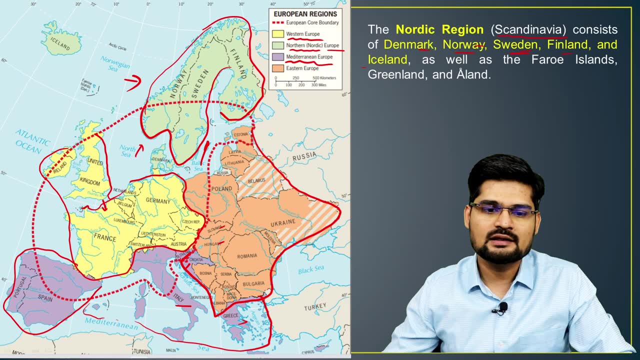 So these are falling under the Mediterranean region And rest is part of the Eastern Europe, if you observe carefully right. So this is where you have Slovakia, Hungary, Bosnia, Serbia, Romania, Poland, Lithuania, Latvia, Estonia, Belarus, part of Ukraine. 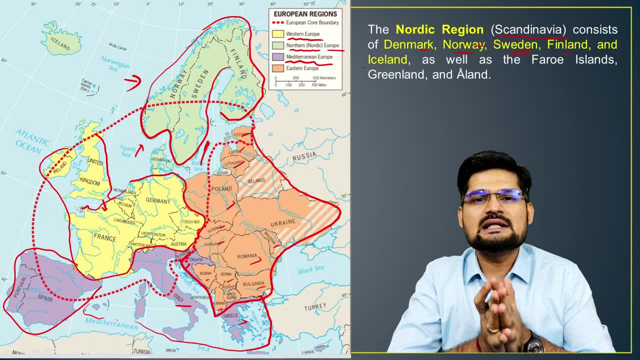 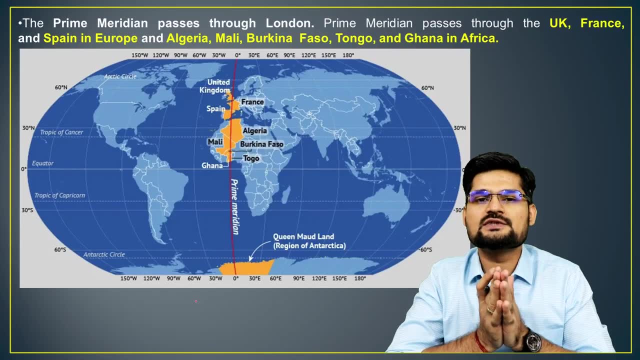 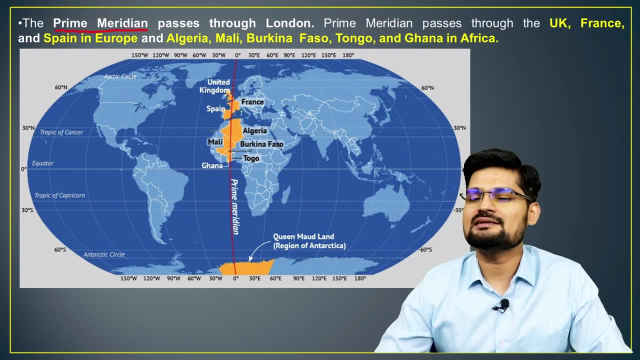 Then you have Moldova, Bulgaria and several others. These are basically the Eastern Europe, right? So this is the regional classification of the European continent. Now If you observe, few more important and interesting information. So, for example, one interesting information is the prime meridian, the zero degree meridian. 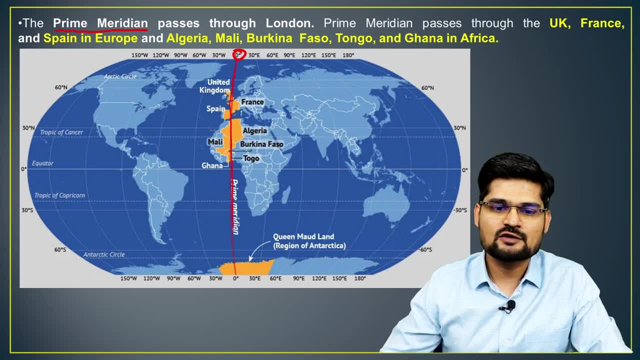 that you observe passes through these particular countries, if you observe carefully. So what are the countries here? UK, France, Spain, Algeria, Mali, Burkina Faso, Tongo, Ghana. So out of this, UK, France, Spain, these are the European countries. 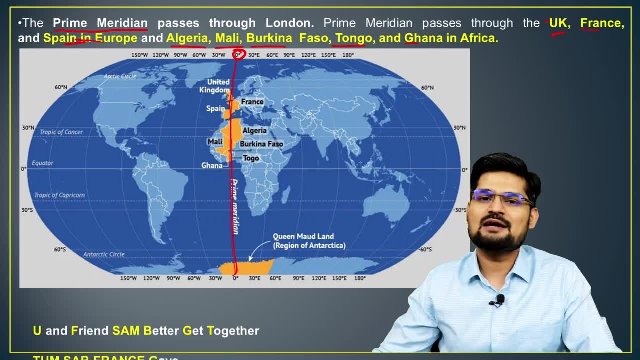 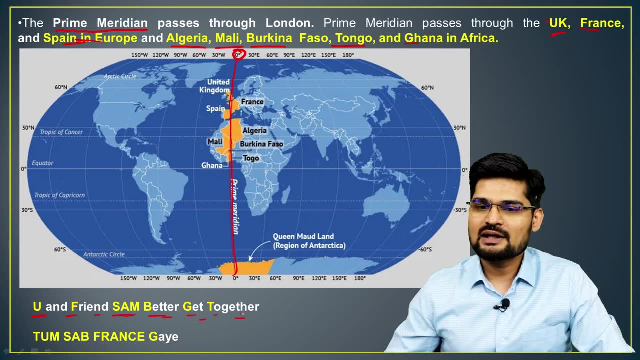 And to memorize these countries. we also can use mnemonics. For example, If you observe U F, Sam, B, G, T. So what is it? You and friend Sam better get together So it's like U F- S. then you have A M, B, G, T. 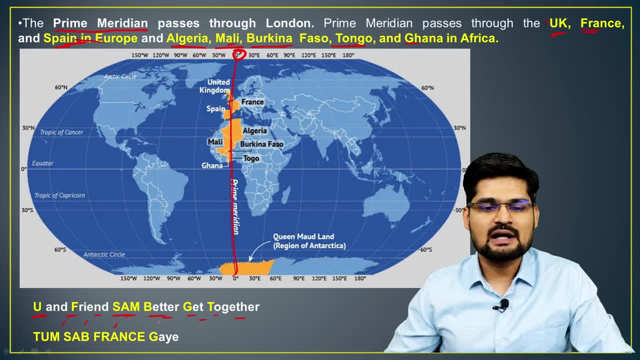 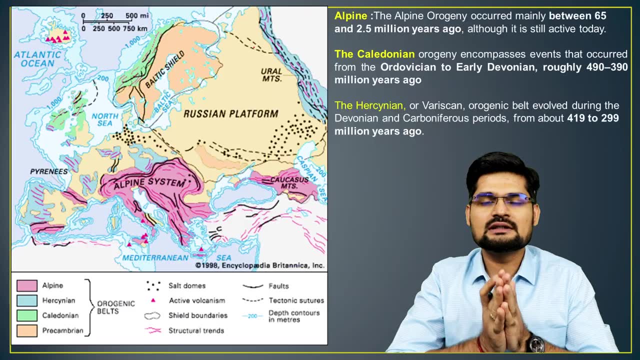 So this is for that, Or in Hindi, if you want to remember it: Tum Sab France Gaye. So this represents these countries, if you observe. So that's the way you can remember, if you want to. Now let's go further and look into the geology of the Europe. 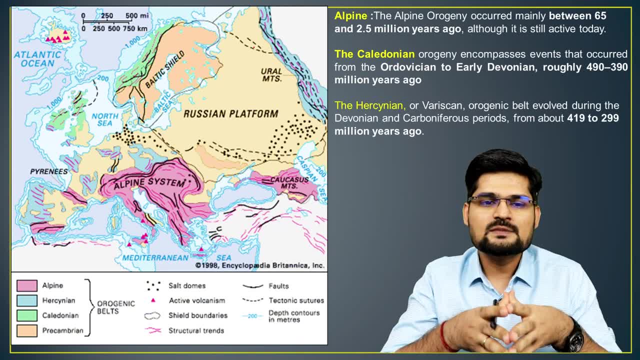 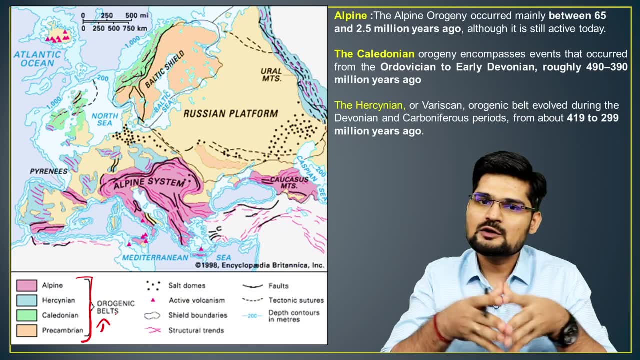 So when we look into the geological regionalization of Europe, we observe that this entire landmass- different types of orogenic belts, means mountain formations- happen and also epigenetic formations that we observe out here. So if you observe, it ranges from Precambrian to Alpine right. 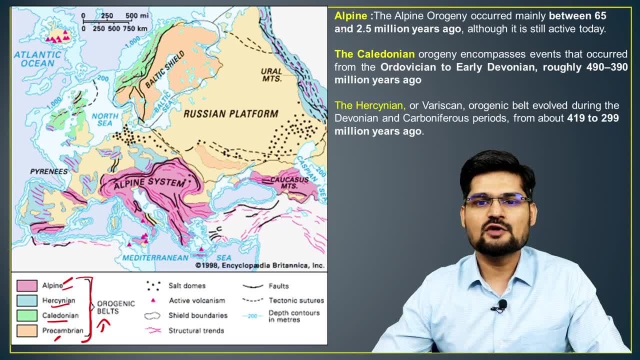 So Precambrian, Caldonian, Hercenian, Alpine belt. So, if you observe, Precambrian is before, 540 million years ago- that we already talked in the earlier lectures also- And after that, if you observe, is these periods: 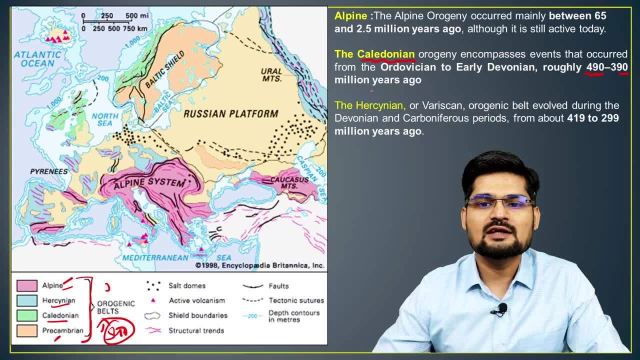 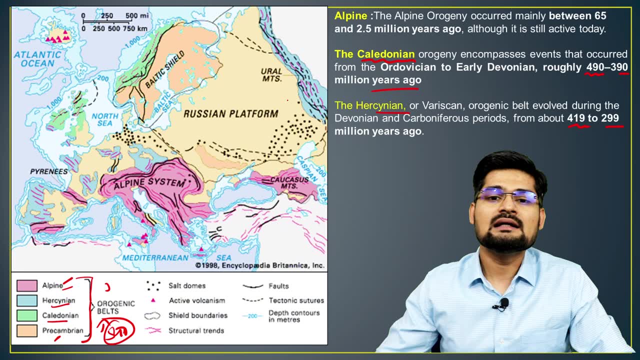 So, if you observe the Caldonian, which is 490 to 390 million years ago, Hercenian- Hercenian is roughly 490 to 299, roughly around the formation of Pangea, And then the latest one is Alpine region, which is 2.5 million years ago to 65 million. 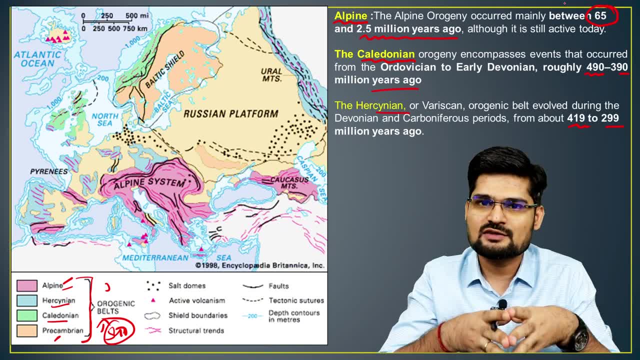 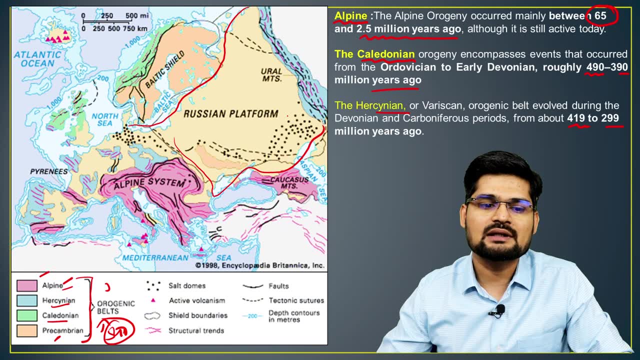 So between 65 to 2.5,. this is the Alpine region of Europe And you can see the color coding as well. So large part of Europe, if you observe, has evolved in Precambrian times. Then this green is your Caldonian, which is part of the Baltic Shield nearby. 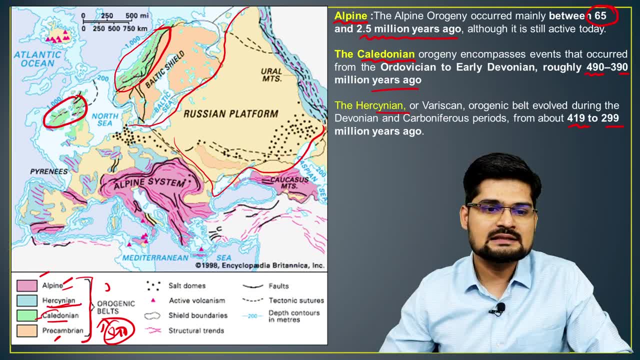 And these islands out here. Then if you observe the Hercenian, these Hercenian are nearby the Oceanic region and the Mediterranean region And in between, this entire pink color that you observe is the Alpine system and Caucasian system right, This is the geological structure of European countries. 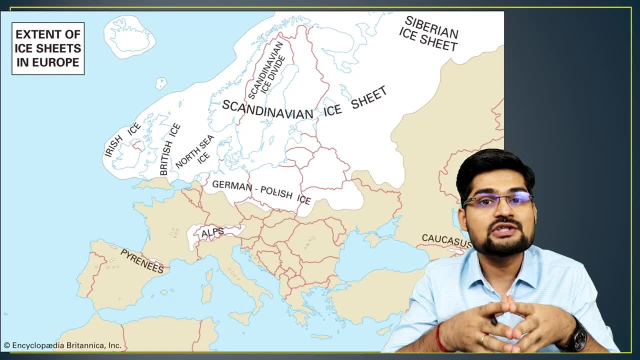 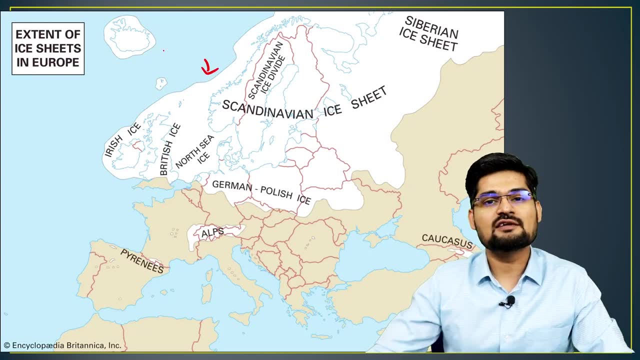 Now, if you observe further the ice age and the extent of ice sheets, And remember it's very important to look into it because this ice sheet and extension gives the landscape that feature, which is majorly glacial landforms that we observe. 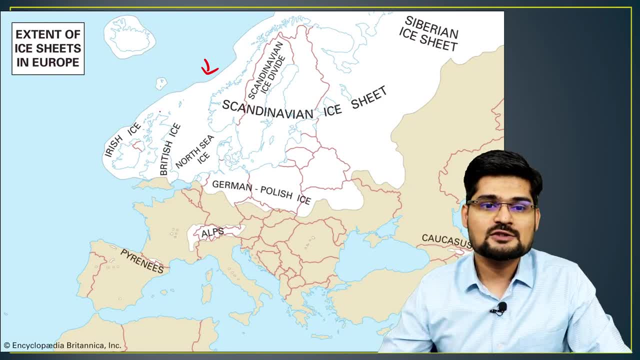 like Norfolk, Norway and fjords and several other features that we observe. So look at these extent of Irish ice sheet, British ice sheet, North ice, Then you have German Polish ice sheet where you have Carpathian and Tatra mountains And we find several glacial landforms out there. 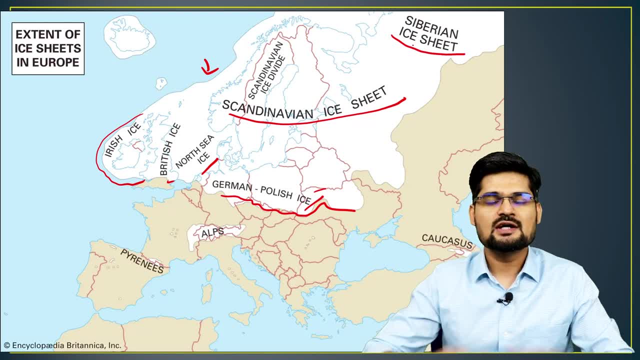 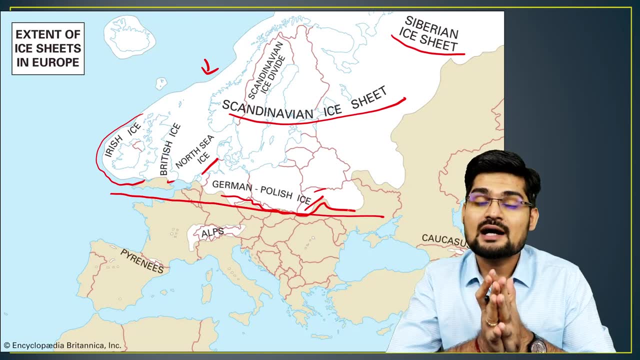 Then you have Scandinavian ice sheet out here and then Siberian ice sheet. So this was the extent. if you observe, almost half or more than half of Europe was covered by ice sheet which started to melt, And then what happened was the flooding nearby, and then water came inside. 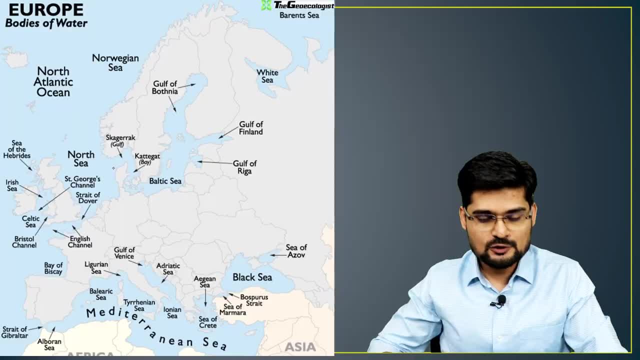 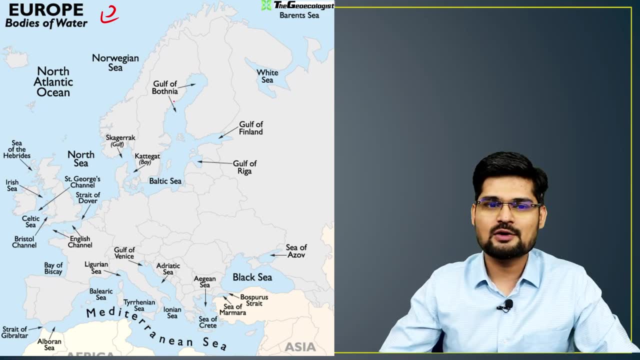 So many seas, many gulf areas you observe here. So to look into that, let's observe another thing. What is it? Europe's water bodies. So if you carefully observe Europe's water bodies, they have an imprint of the last ice. 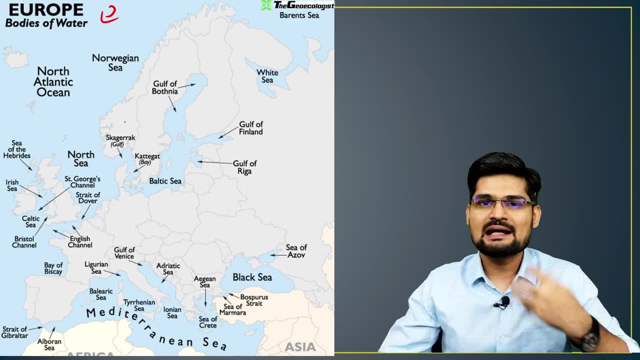 glacial age, right, So glacial maximum, and then the retreat and then the water intrusion inside the land, So leads to a lot of gulf formation. So if you observe from north Barents Sea is here Then you have the White Sea, this gulf area. 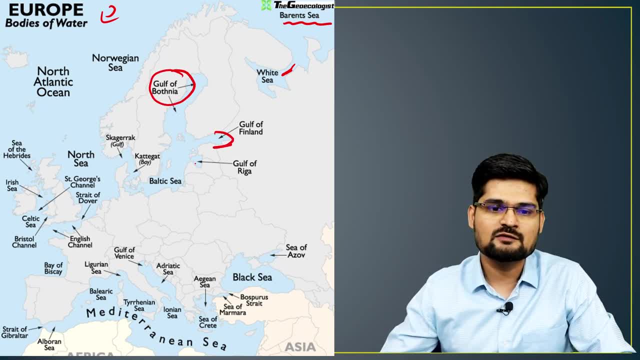 Then you have Gulf of Botnia out here, Gulf of Finland out here, Gulf of Riga out here, And this is the Baltic Sea right. Then you have the Kattegat Bay, Then you have the gulf here, Skagark. 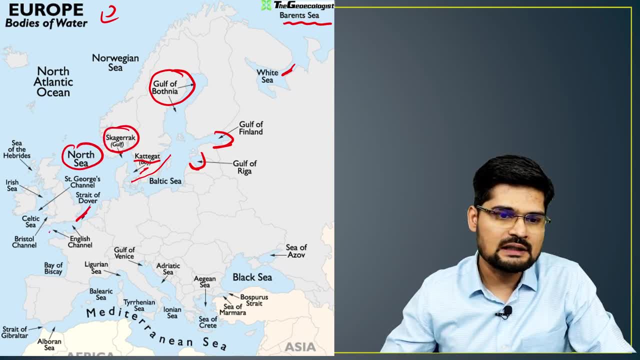 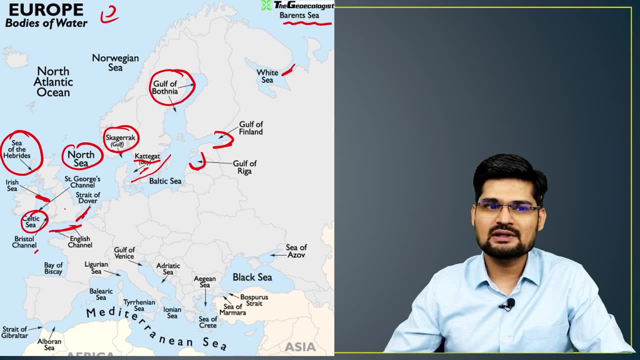 Then you have North Sea. out here, right Here you have Strait of Dover, English Channel, Celtic Sea, Bristol Channel. Then you have Irish Sea, Sea of the Hebrides. These are the important areas near Iceland. You have the obviously North Atlantic Ocean part of it. 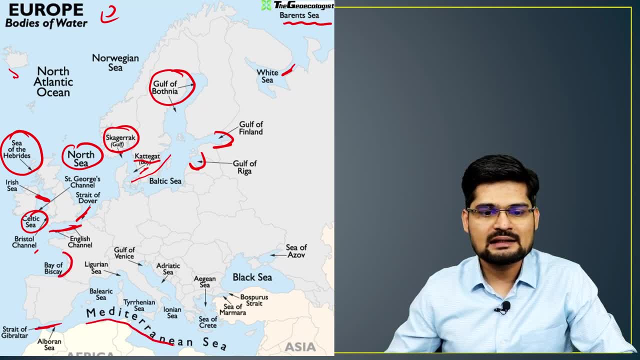 Then you have the Bay of Biscay, Strait of Gibraltar, the Mediterranean out here, And Mediterranean is further branched into several gulfs and seas. Observe carefully. You have the Balearic Sea, Ligurian Sea, you know this is Gulf of Venice, here Adriatic. 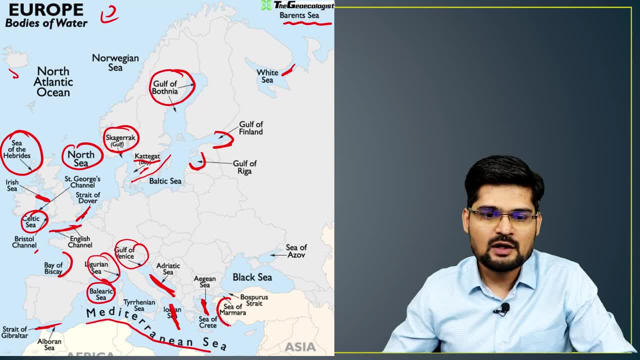 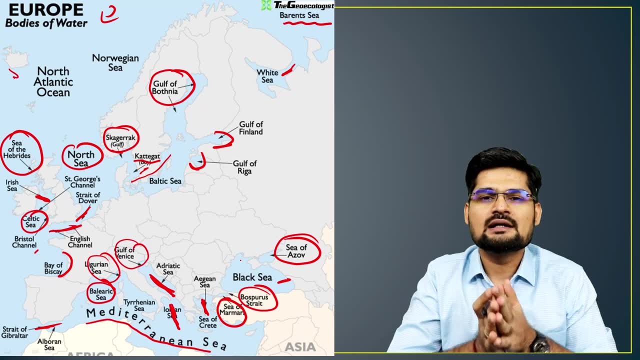 Sea, Aegean Sea, Ionian Sea, right Sea of Marmara is here. Then you have the Bosporus Strait, Black Sea, Sea of Azov. All these numerous water bodies are the representative of the fact, of the geological structure. the 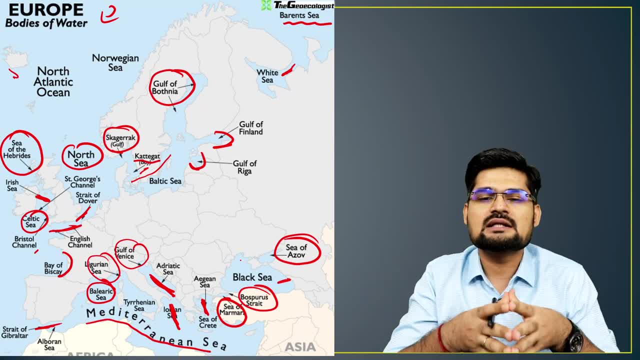 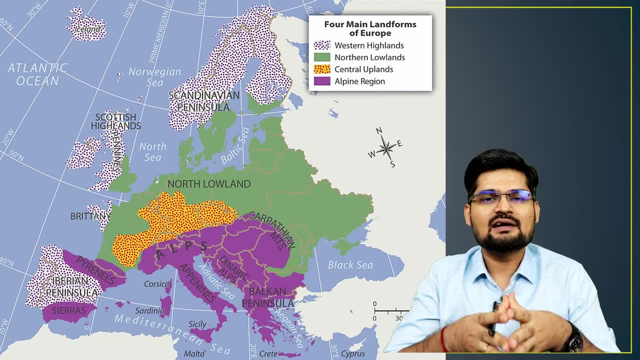 Plast, Glacial Maximum and several other features which are there as part of geomorphology in today's world. Now, if you observe carefully, The geomorphology of Europe Can be divided into four major classes of landforms. So four major classes, if you observe, is Western Highlands. 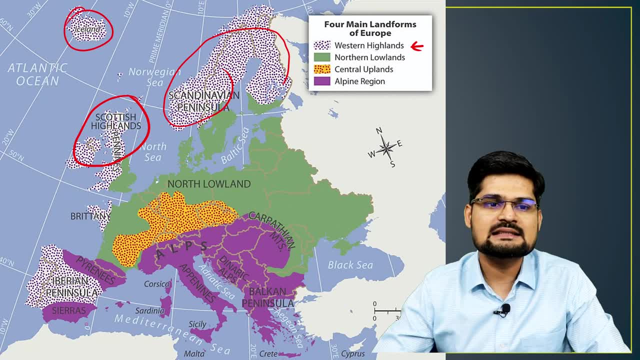 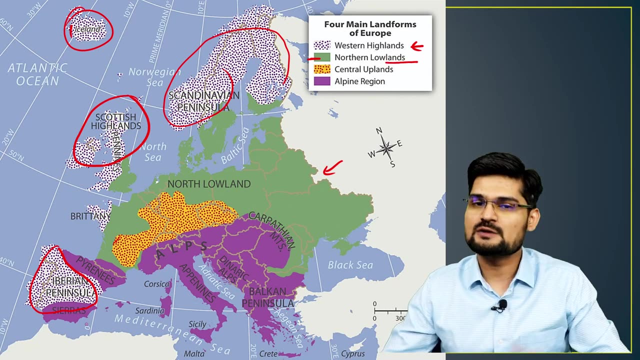 So these entire Scandinavian countries, Scottish Highlands, Iceland, Then you have the Iberian Peninsula region. These are part of the Western Highlands. Then, if you observe the green patch out here in the center, This is purely the Northern Lowlands and Plain Areas, which is very huge area and also has 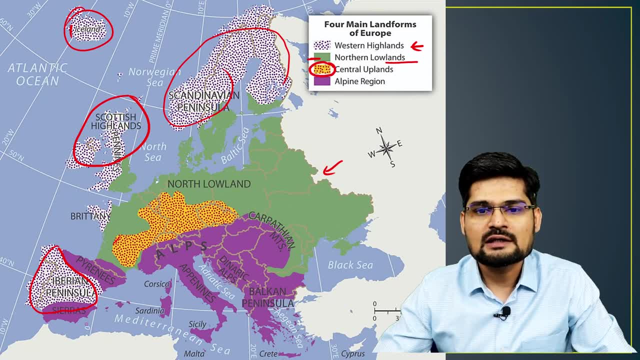 a huge population base. Then you have this yellow and red dots which you see is central, Central Upland area, which is just the nearby extension of the Alps. right, This area is your upland. And then you have the major purple patch of Alpine region out here. 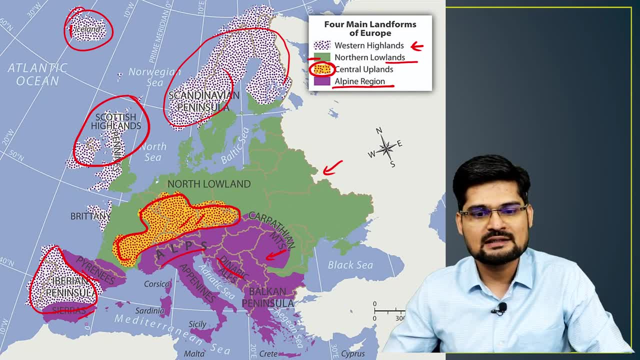 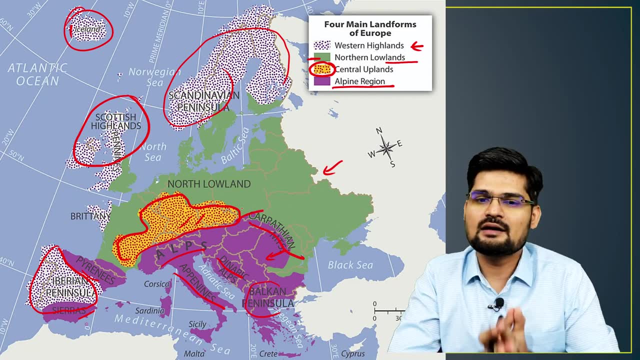 If you observe carefully the Pyrenees, the Sierras, the Alps, the Dinaric Alps, the Apennines, then you have Vulcan Mountains right, Carpathian Mountains, Tatra Mountains- all those mountains are part of our Alpine region. 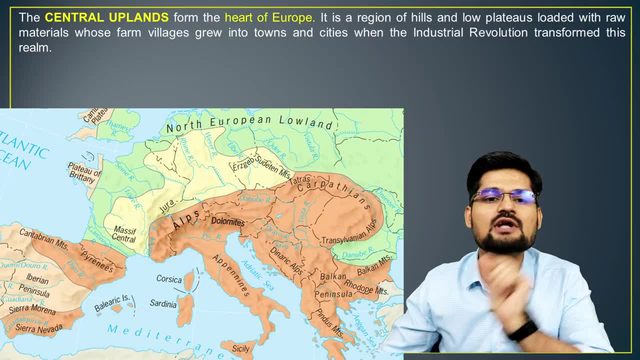 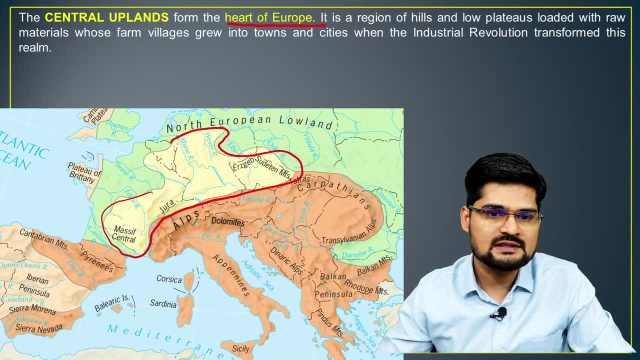 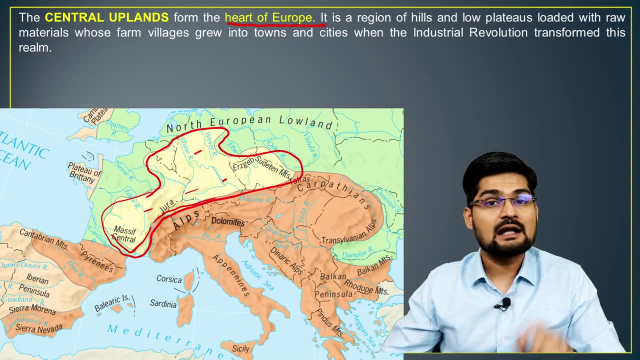 Now further, if you go, let's look into one by one. The central upland forms the heart of Europe. So this is the central upland area where you observe these particular regions here and it is endowed with several river system, You observe Rhine River and other river and central massive Jura Mountains. 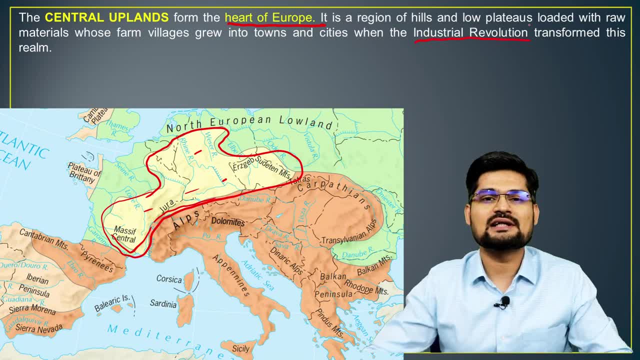 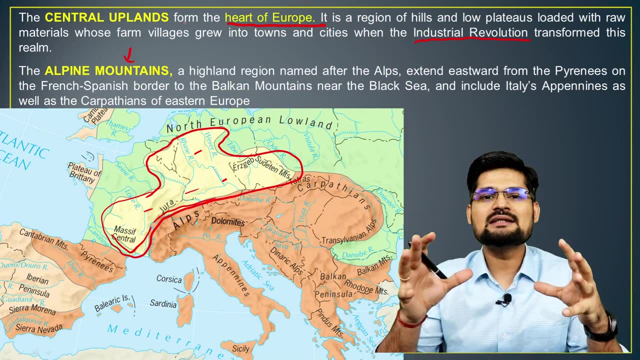 And remember this heart of Europe was the seat for industrial revolution. It has a lot of minerals and industries. Then further, if you observe, is the Alpine system, the most famous one in the world. So Himalayan system and Alpine system are the most famous mountain systems because they 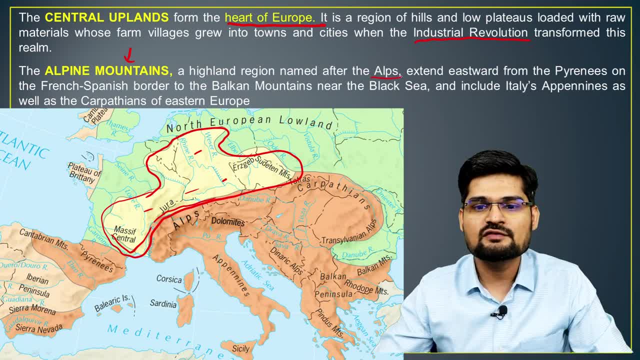 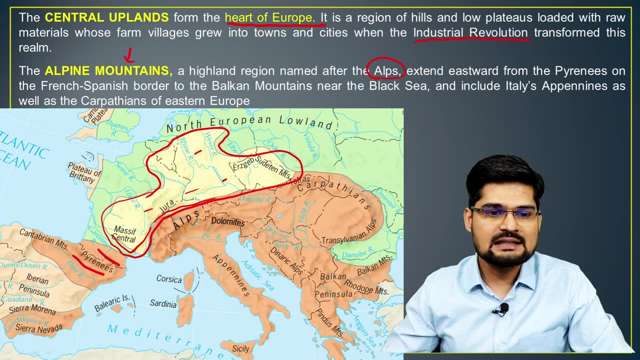 are still growing, There is still movement And Alps is one feature, One feature which is most famous feature in European geomorphology. And if you observe further, Pyrenees are here, then you have Sierras here, Dolomitic Alps. 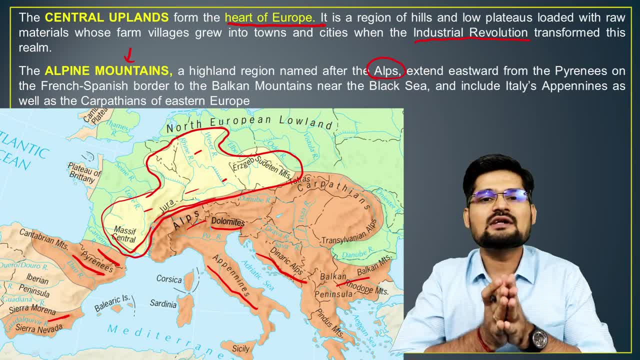 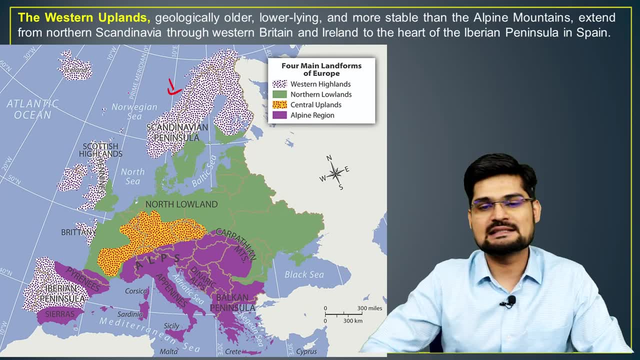 then you have Apennines here, Dinaric Alps, here Vulcan and several other mountain chains in the Alps. Now, if you observe further the Western uplands, which is part of the islands basically, and these Western uplands are geologically older systems, lower lying and more stable than 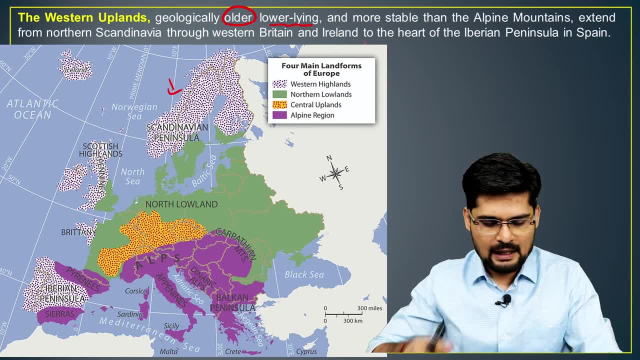 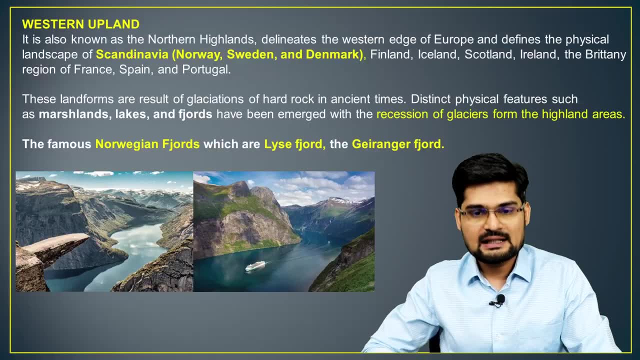 Alpine mountain system. right, The older formations, they're more stable and they're part of, majorly, the Iberian Peninsula and these particular islands and the mainland part here right Then, if you observe, the Western upland has certain very interesting glacial features. 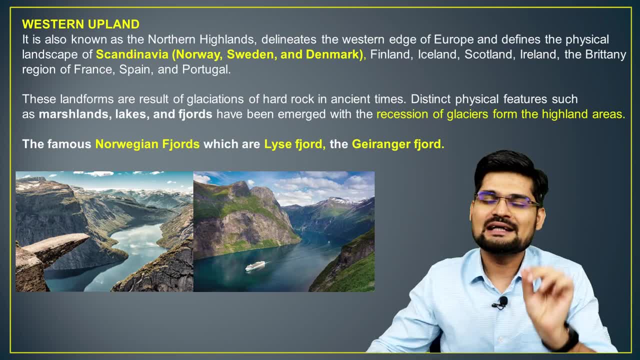 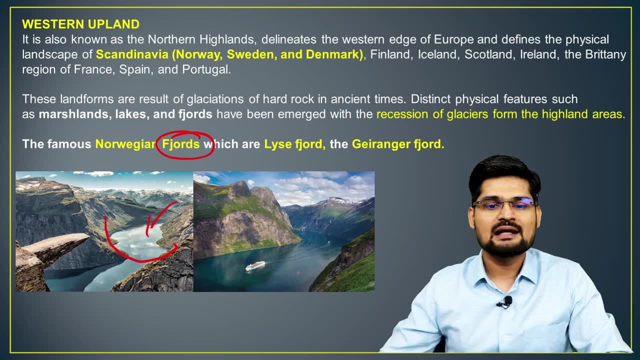 if you observe- and I'm sure you have learned about this before in glacial geomorphology as well- by the name of fjords. So these are the U shaped valley carved by the glaciation earlier, and now the sea water is intruded because of rise of sea and then it is now navigable. 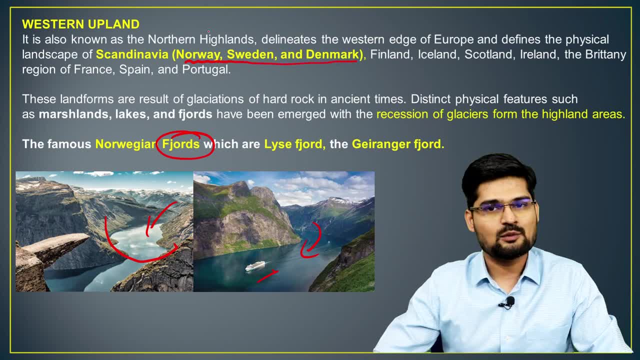 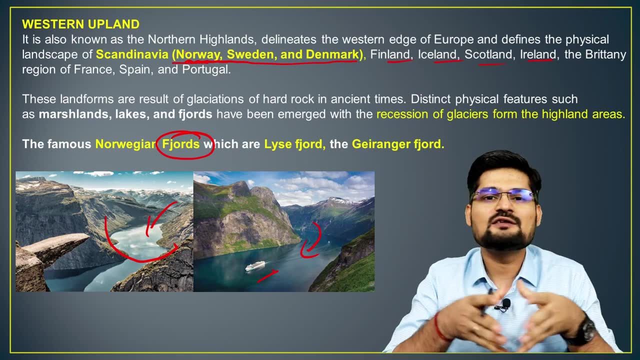 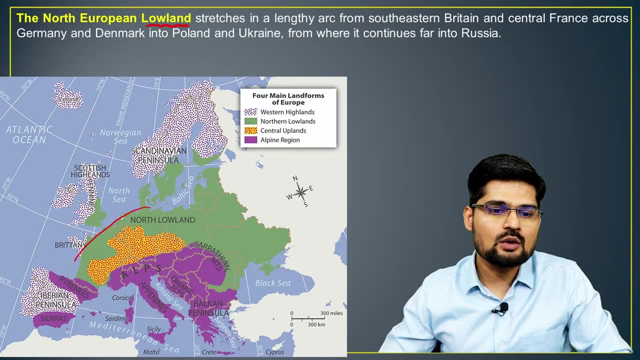 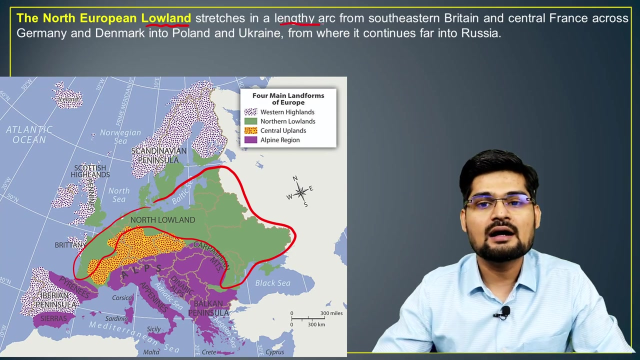 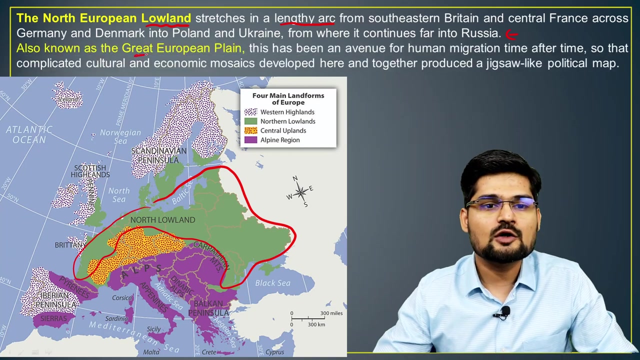 So this is found. You can see that the defenses of these Black Sea islands throughout the înn fail州, the, and then further, what is the importance of it? the great european plain, as we also know, is the major avenue for human migration time to time. 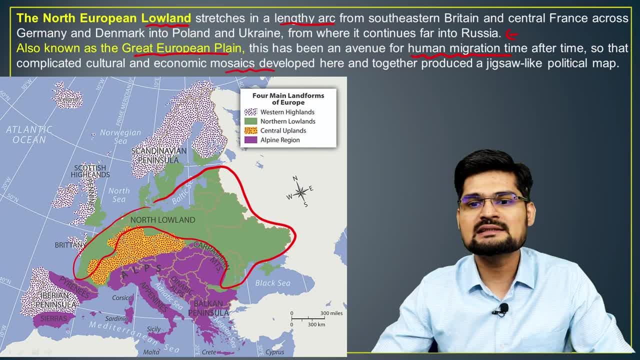 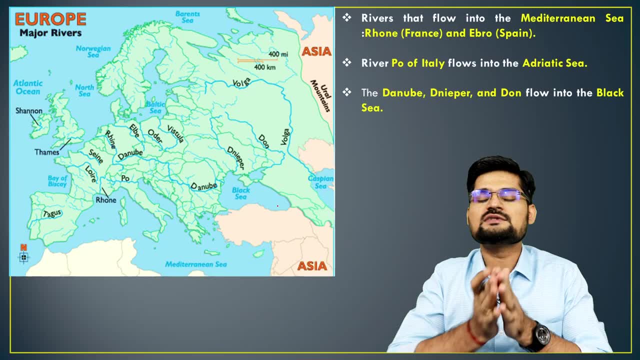 and it has a congregation of human cultures, economic mosaics, and therefore it's like a jigsaw fit that provides and has been changing for several decades now. now, if you observe further the major rivers of europe. so, of course, because of the geology and geomorphology numerous river, 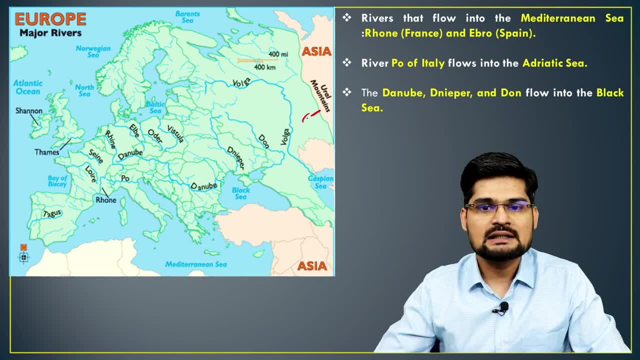 systems are available out here. so if you observe carefully in the map, these are the rivers, so river that flow in the mediterranean, you can observe rhone and elbro here. if you observe the rhone and elbro in the spain and here this portion, then you have po of italy falling in the adriatic sea out. 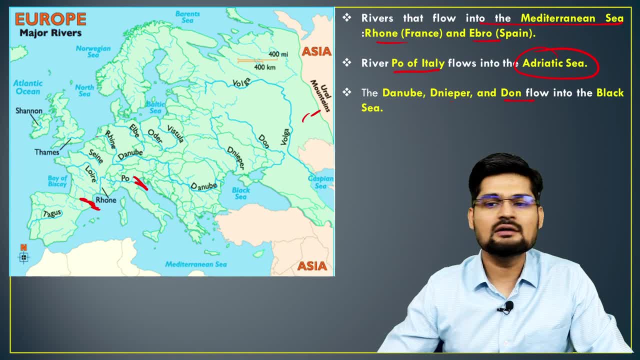 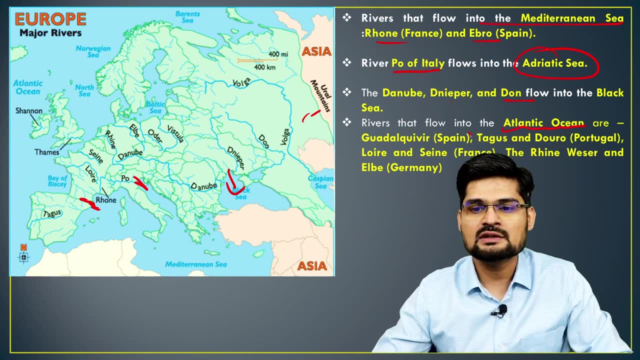 here this is adriatic sea. then you have danube, denpa and don river in the black sea. they form here this particular, and then, if you observe further, there are other rivers that flow in atlantic ocean, the rivers of spain, portugal, france and germany. so there are rivers which flow in the 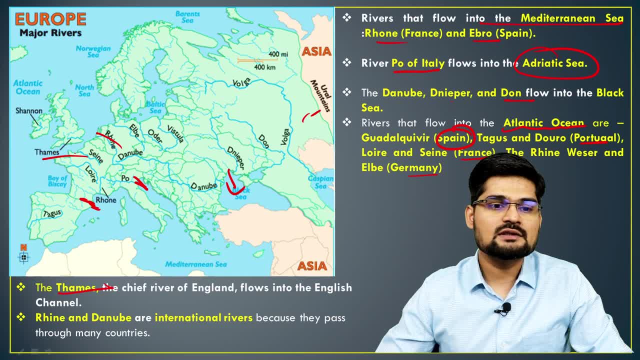 atlantic ocean as well, and then further the thames river, which is very familiar to you, and then, if you observe further, the thames river, which is very familiar to you, the thames river, which is very familiar to you, and then, if you observe further, the thames river, which is very. 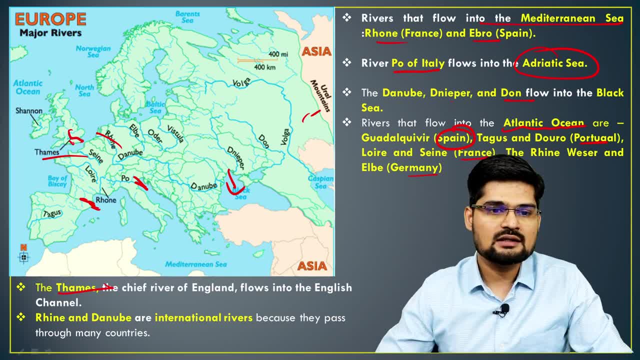 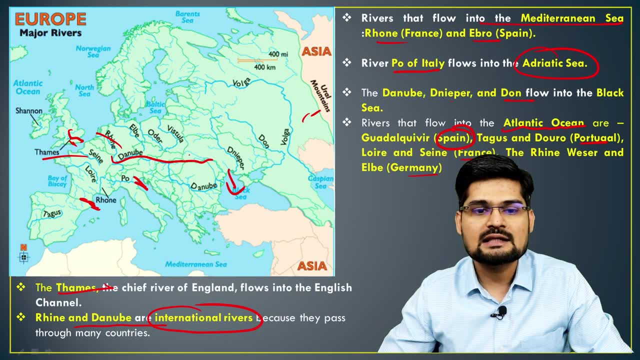 famous river of england and it is flowing in the english channel out here. then you have rhine and danube, which is majorly the international river which cut across many countries. they are not in the single country right, so these are the river which are across the international borders and 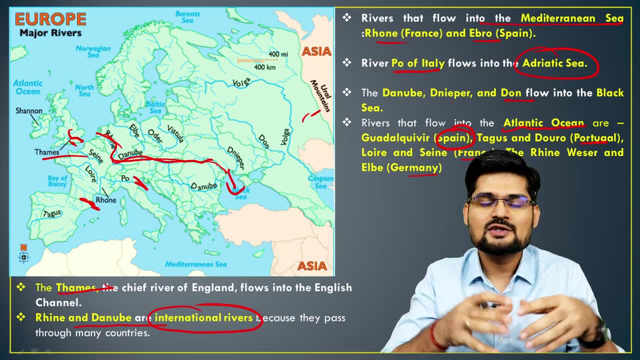 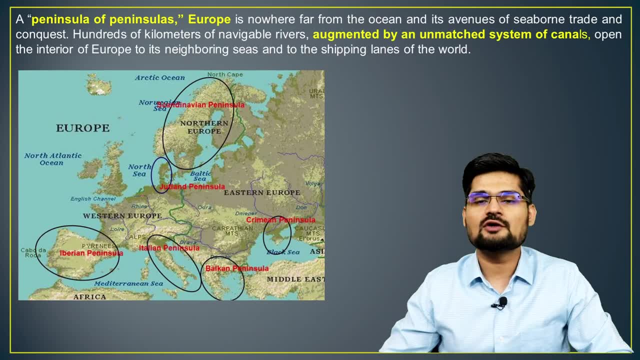 now, if you remember the integration of europe, that is european union. so these rivers are flowing across the countries and integrating them through their channel links. that's important. now if you further observe that europe is not just a continent, it's a peninsula itself, and within that peninsula it has several other peninsulas. so if you observe, 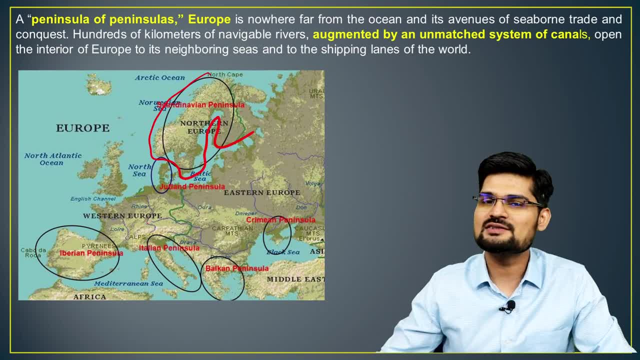 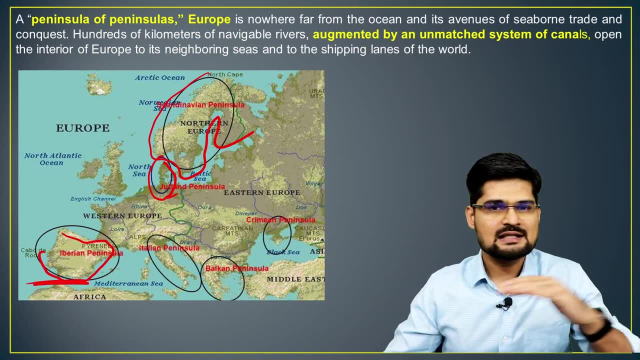 northern europe, part scandinavian peninsula. this is one peninsula. then this is north sea and this is jetland peninsula. then you have iberian peninsula. of course this is straight of gibraltar that separates africa. then you have the italian peninsula, then you have this balkan peninsula. 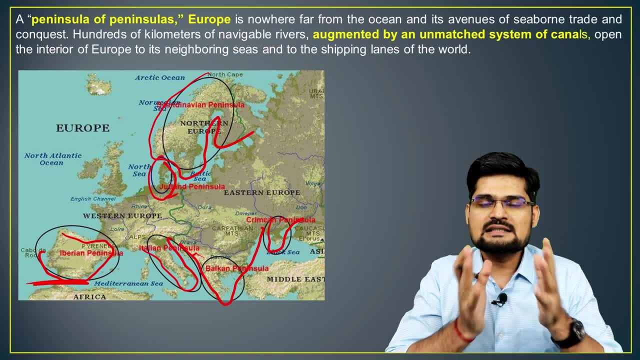 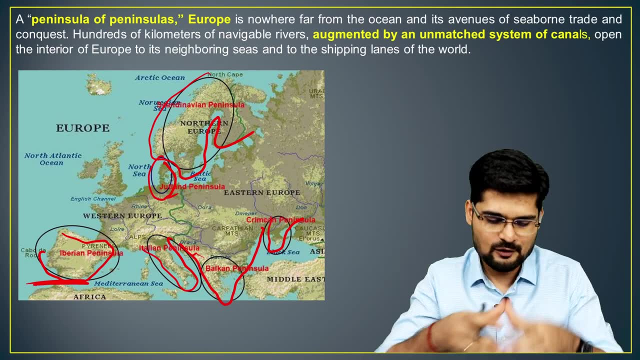 right crimean peninsula. out here, and this is what we say- is that europe is combinations of several peninsulas and augmented by several canals and people of different backgrounds, river system that we observe. now let's look into one of the major systems that divides asia with. 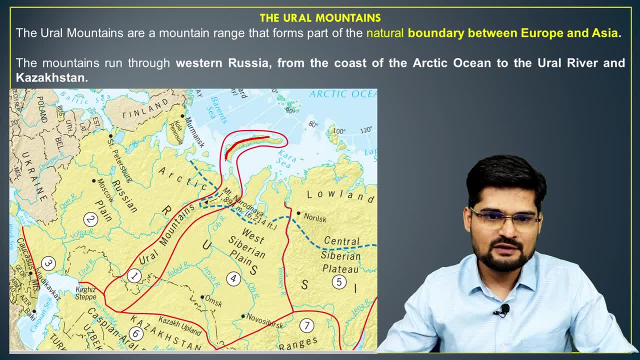 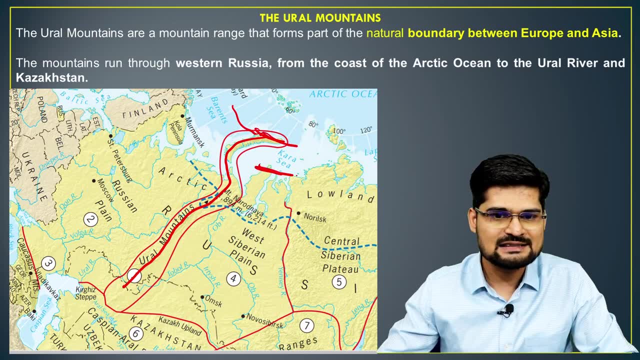 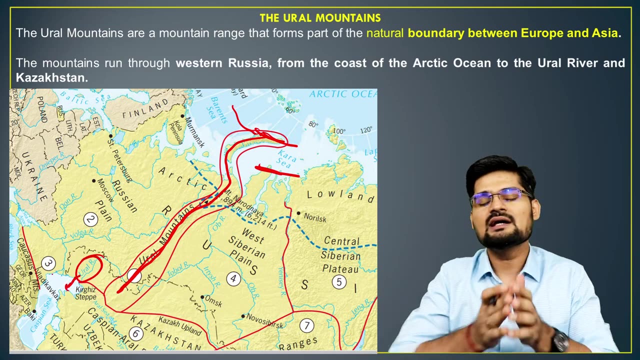 europe and that's ural mountain system. so if you observe carefully, this mountain system out here, rural mountain system right from almost the barren to sea arctic circle, this kara sea out here to this system goes down south to kazakhstan. here you have the ural river right which falls into the 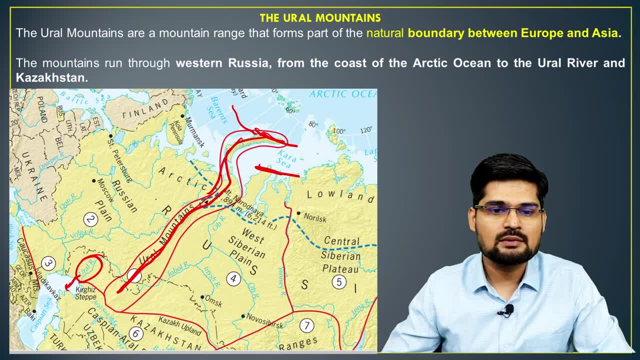 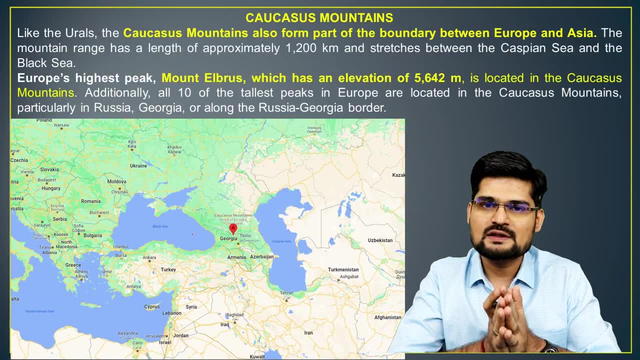 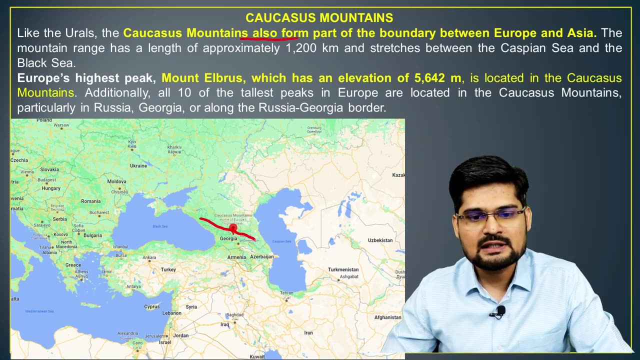 caspian sea. so this is the main mountain system that branches the europe from asia right and then further. there is another mountain system that we already know as caucasian mountain system, the caucasus. so caucasus mountains form the boundary between europe and asia, and this is where the 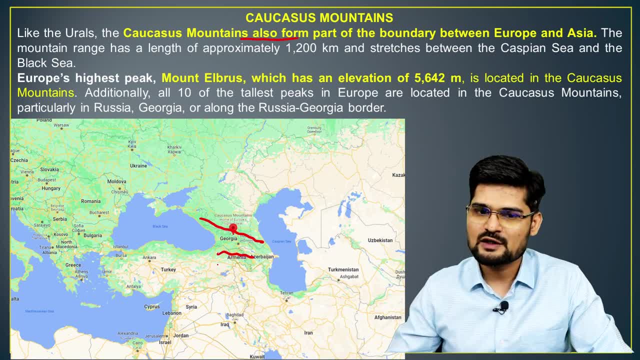 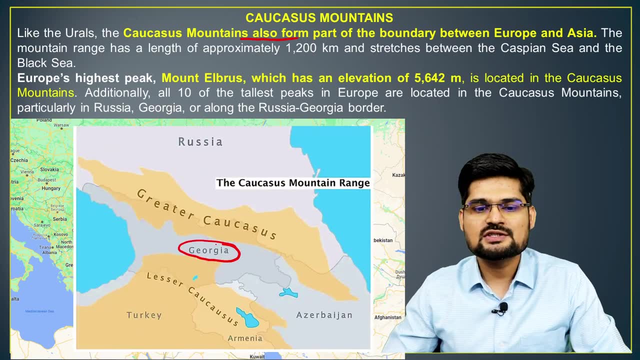 greater and the lesser caucasian mountain systems are available between the black sea and the caspian sea, and the countries nearby, if you observe, is majorly georgia. that falls between these caucasian mountains, the meridian mountain system and the caucasian mountain is the caucasian. 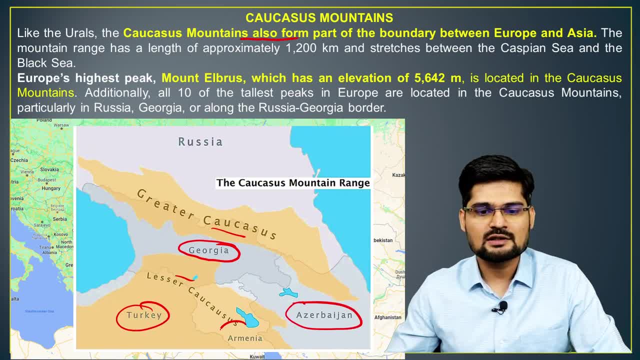 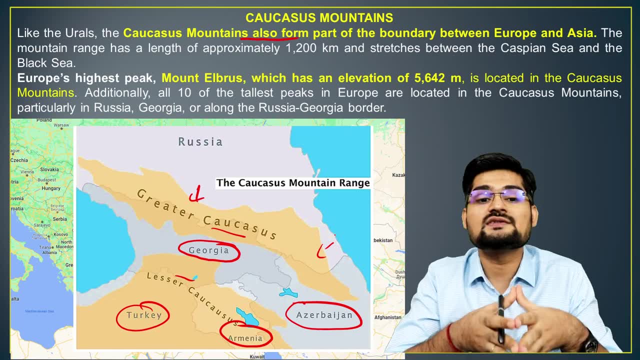 mountain systems. then you have the Azerbaijan, then you have Turkey, out here Armenia, out here right, and then in the north is Russia. so these are the locations which are important if you talk about Caucasian system, and remember Mount Elbru is the greatest mountain in this system, which is 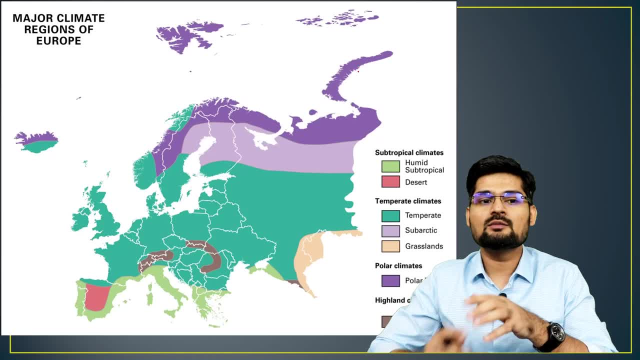 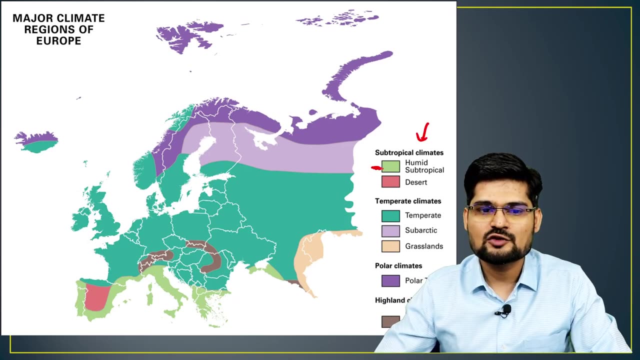 5,642 meters. and remember one more point: that major climate if you observe in Europe is the feature which is part of the geoclimate itself, because it is in temperate to subpolar belt, so you have these particular climates available. so look this: green patches, if you observe in certain 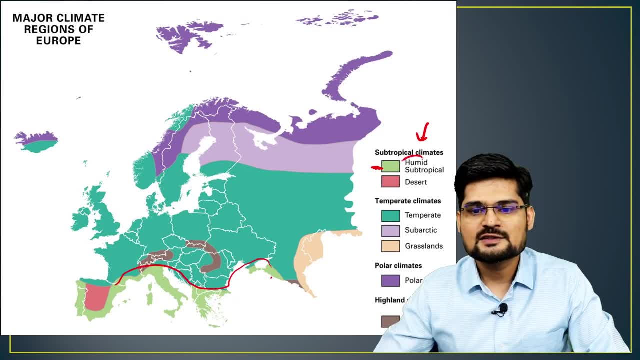 areas down south. the Mediterranean part, if you observe, is humid, subtropical. then if you see the red ones, basically the desertic conditions and then temperate climate, which you observe is the major climatic zone in the entire European system, then you have the subarctic system that is near. 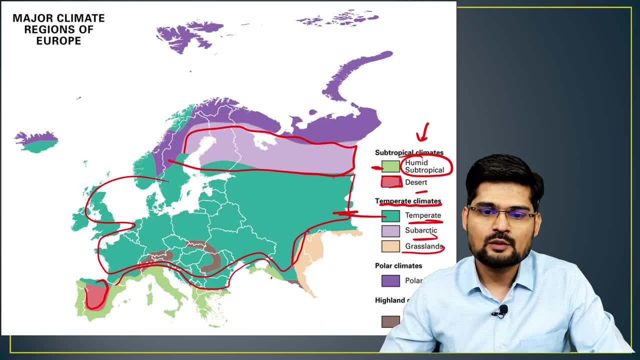 arctic, this portion, and then you have the grassland system which is out here in the eastern Europe, this portion, and then you have the polar tundra, which is close to these particular areas, which is the polar areas, parts of Iceland, parts of Finland and other areas. then further, if you observe, is the highland that varies with altitude, which is part of. 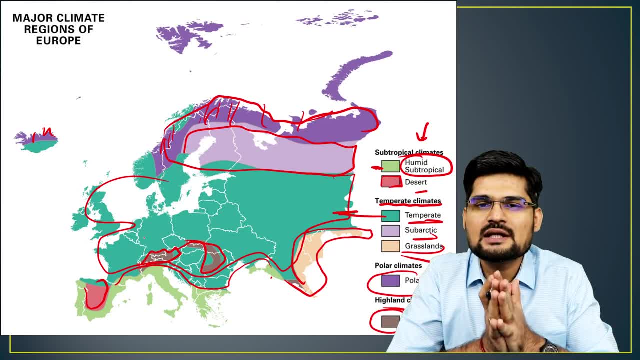 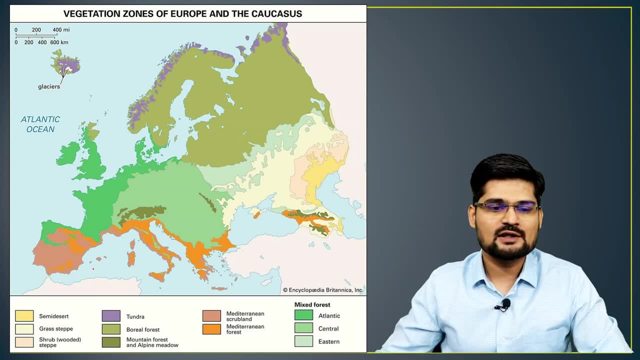 the Alps and adjoining system. so this is how the major climate of Europe varies. further, if you observe the vegetation zones, it's a representation of the geoclimate itself. so you can observe right from the tundra to Mediterranean to mixed forest. everything is available in Europe and you can see. 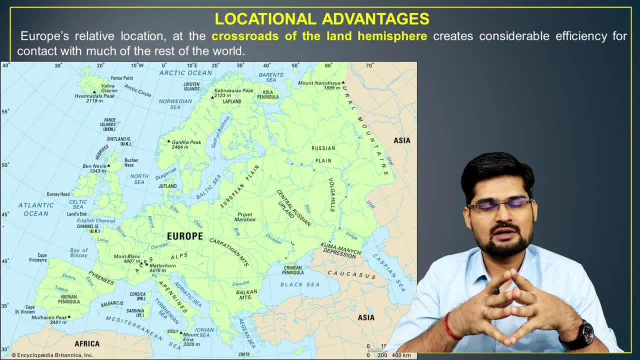 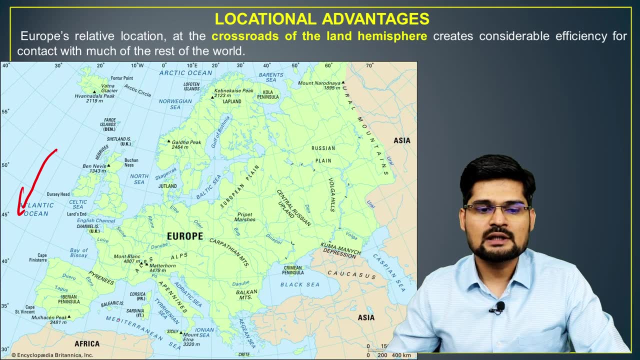 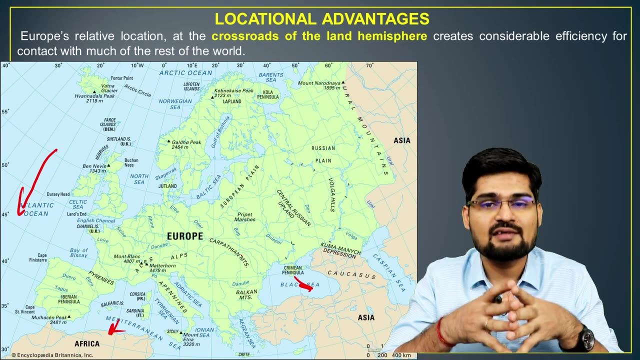 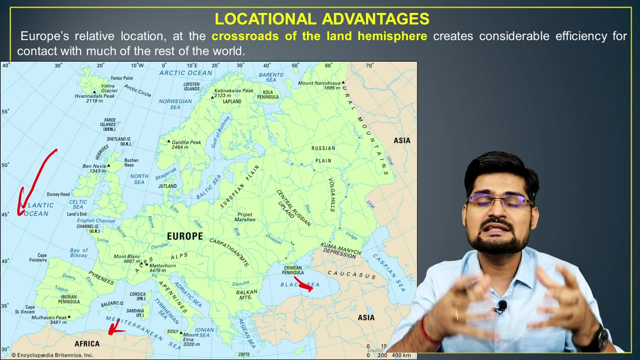 the biggest advantage and that's why Europeans have been the seat of the modern civilizations, the seat of industrial revolution- the Greeks and Romans until present. they are leading the world in forms of industrialization, in terms of knowledge and so on several other fields. so locational advantage is something that we also discussed in the playlist. 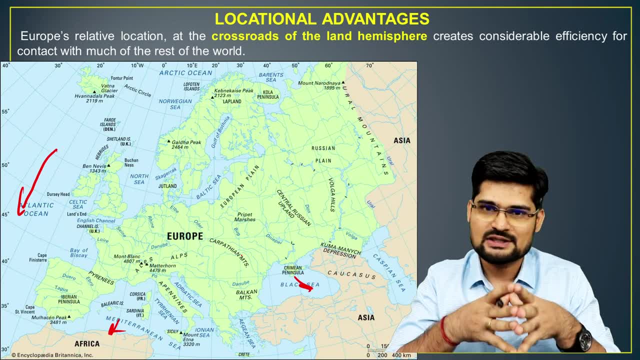 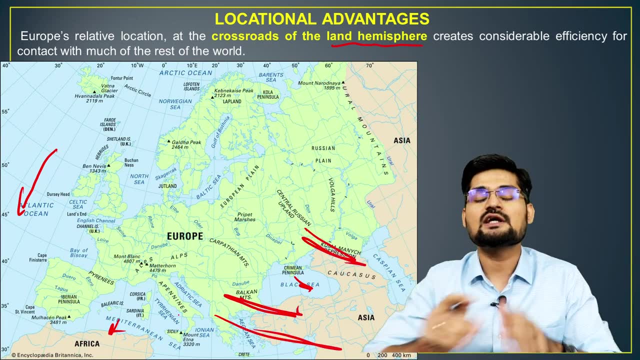 of geographical thought as well. if so, if you have not watched it, you can go there and watch it again. now, this is called the crossroads of land hemisphere and this connect, if you observe, is something which is very important. the europe and asia connect, so this is one advantage that 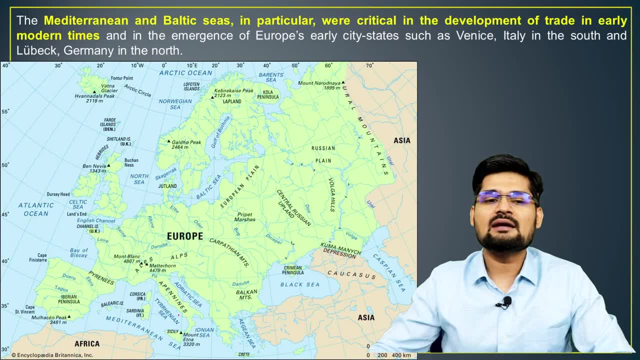 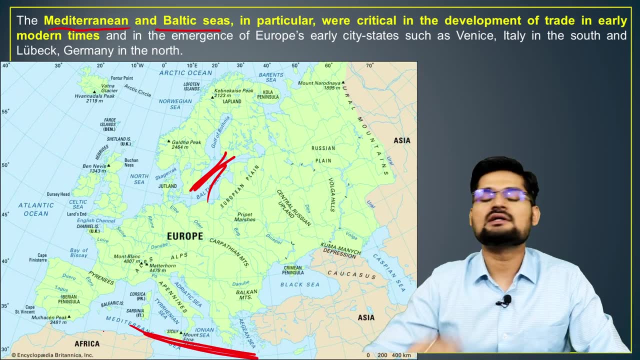 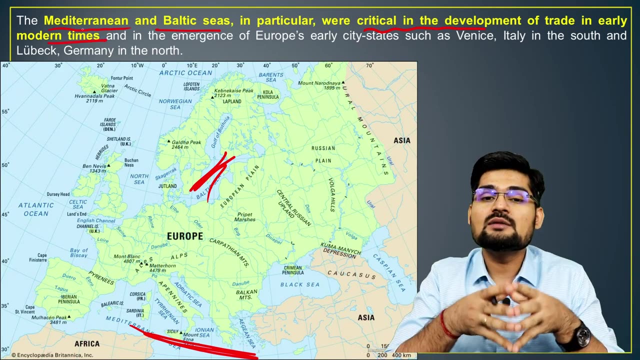 we talk about then further, if you observe mediterranean and baltic seas, these two seas, the mediterranean seas and the baltic sea, these particular, this particular seas in particular, were critical in development of trade in early modern times and, if you remember, these were the mercantile. 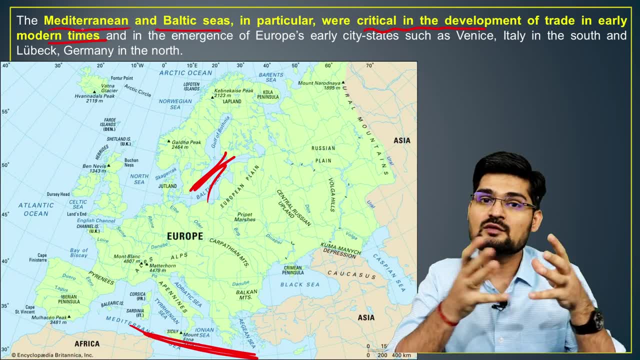 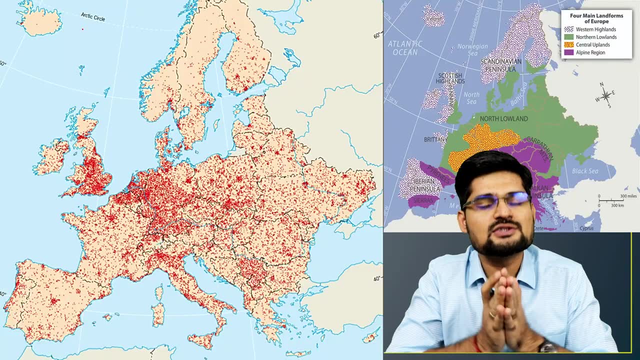 states which flourished since the middle ages and even before, and then we had a lot of development in terms of navigation. that's important. then if you observe the population geography of europe, because of the lowland, highland system, mountain and then valley system, the population is: 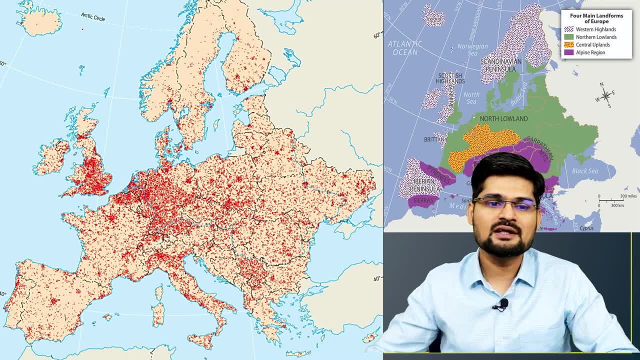 suitable for the population of europe. so if you observe the population geography of europe, sporadically or haphazardly distributed, if you observe carefully. but major concentration is the uk, then you have this area of germany and france out here, some in italian alps and nearby areas. 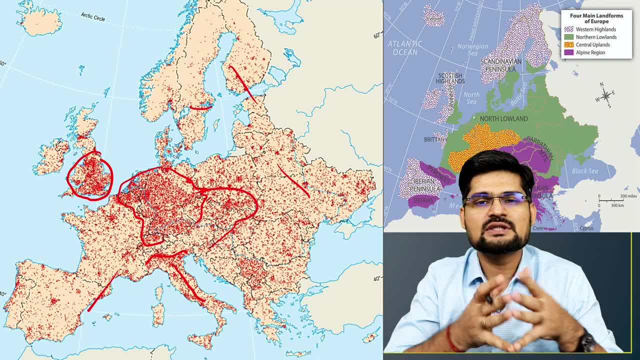 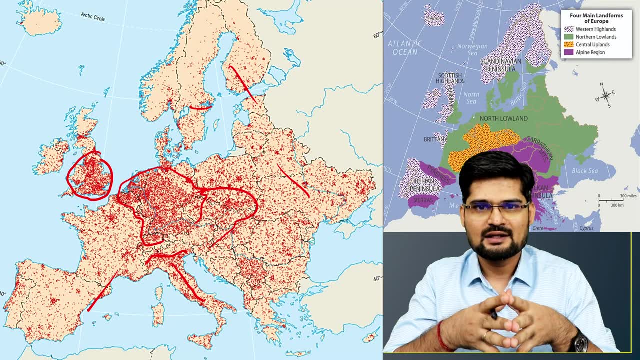 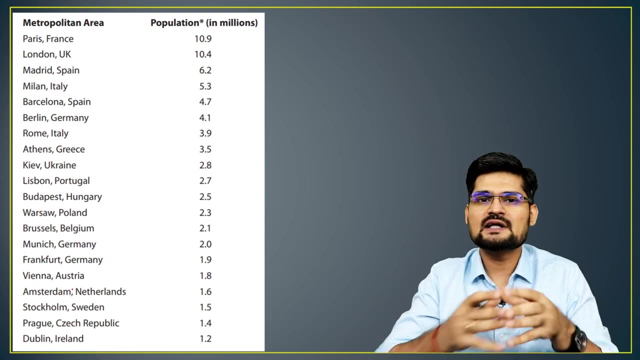 but most of the other areas of europe, especially northern area, northeastern area and northwestern areas, are not well populated. they are very sparsely populated, right as you can observe on this map as well. then, further, the data of this particular population in terms of cities also shows that. 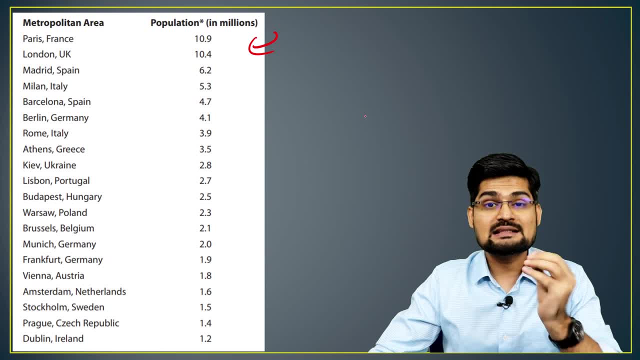 metropolitan areas are very sparsely populated. so if you observe the population geography of europe, you can see that the population of europe is very sparsely populated and the population areas are also not as heavily populated as some cities in india or in other parts of asia. right, look here. paris is 10.9. 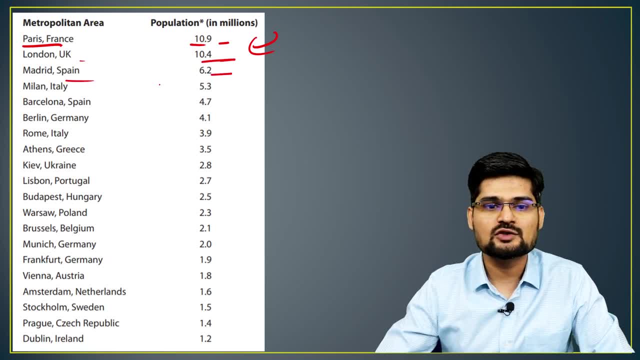 million, then london is 10.4 million, madrid is 6.2, milan is 5.3, barcelona is 4.7, berlin is 4.1 and then rest are not even 4 million. so this is how we observe carefully the list of cities, the major. 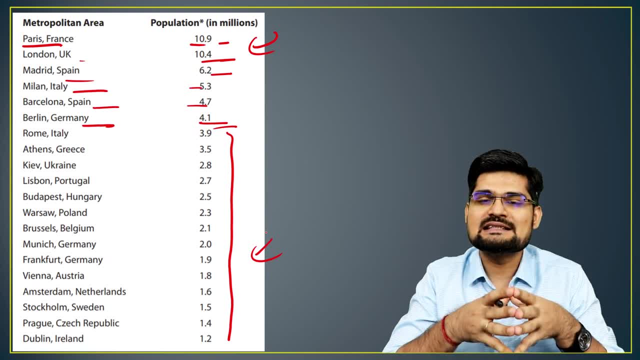 cities and their population. so what does it say? most of these cities, most of these countries in which these cities are there, they are highly developed in terms of population. so we observe they are highly developed in characteristics, right? that's very important to understand here because of low population base and high level of resources. so, per capita resource availability, if 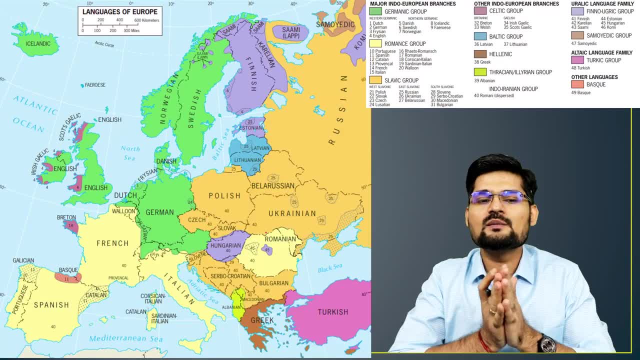 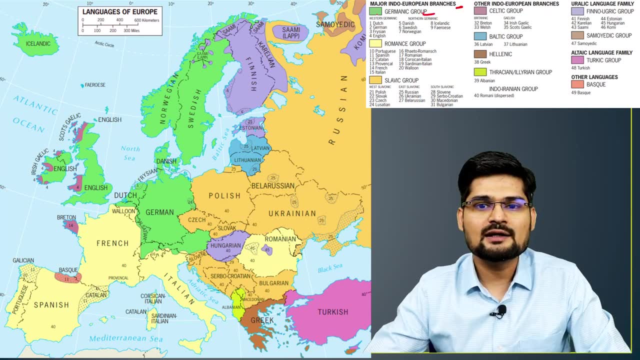 you observe, is very healthy in these countries. now, if you observe the languages, so languages being part of the human cultures. now, if you observe the major european branches, germanic group is completely green in nature. if you observe, so norwegian, swedish, german, dutch, english, right, these are part of the germanic group. then you observe romance group, so you have the portuguese. 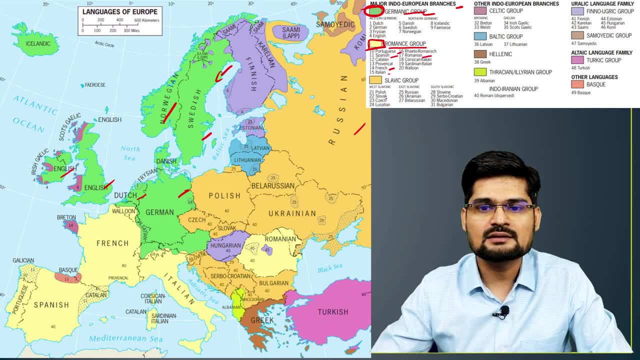 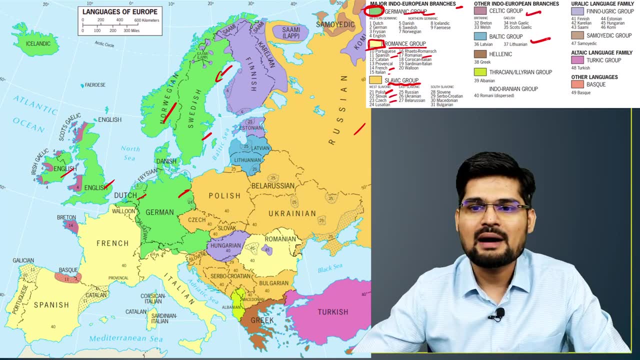 spanish, then your french, italian, romanian and others. then you have salve group. so salve group is observed here: polish, slovak, czech. then you have celtic group, baltic group, hellenic group. several groups are available out here, as you can see, and you can pause the video and look for yourself. you. 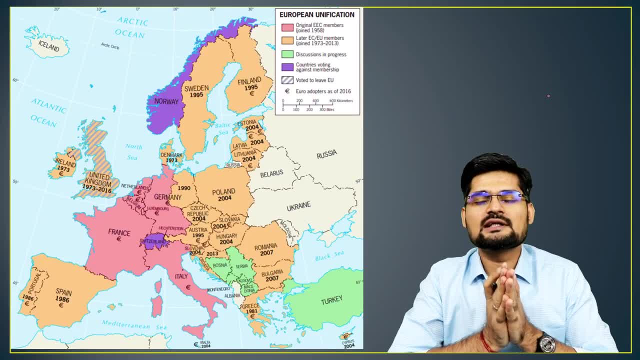 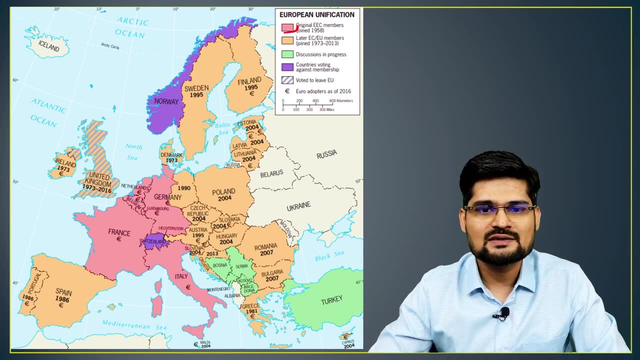 can draw the map yourself as well. now, if you observe further, the unification of europe, the european union, that we say, is a very interesting characteristic, right so right. from this color coding you see the first ones till 1958.. this area was the most important part of the european. 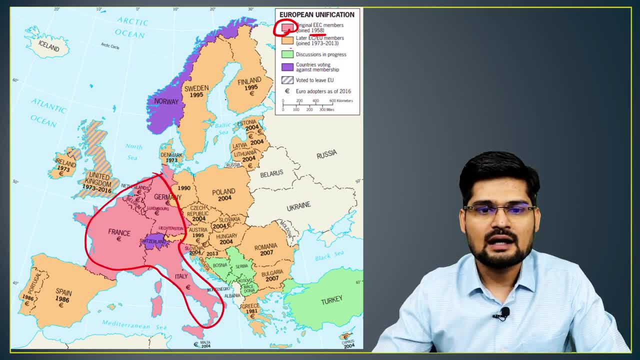 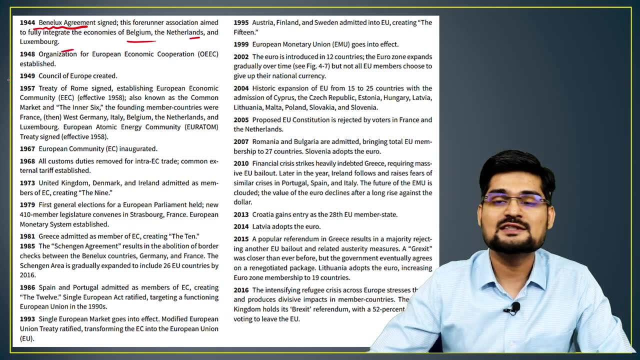 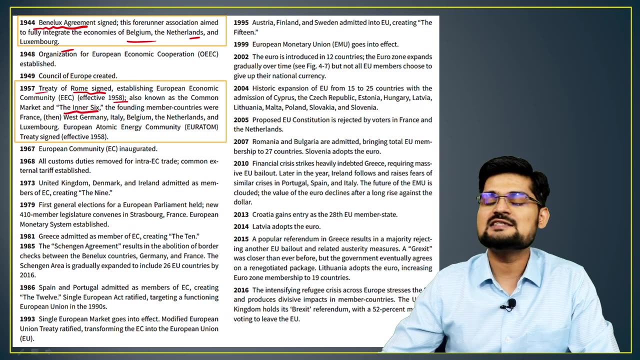 union. it was the first area which got unified. then later other areas got unified and there is a history to it, right from 1944, the ben lux, belgium, netherland and luxembourg formation. right then we have the treaty of rome, signed in 1957, 58, where the inner six countries joined it. 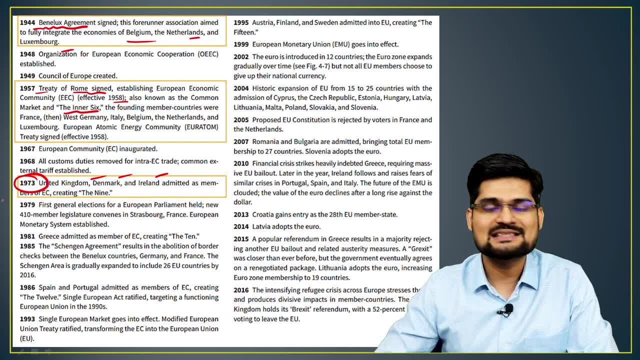 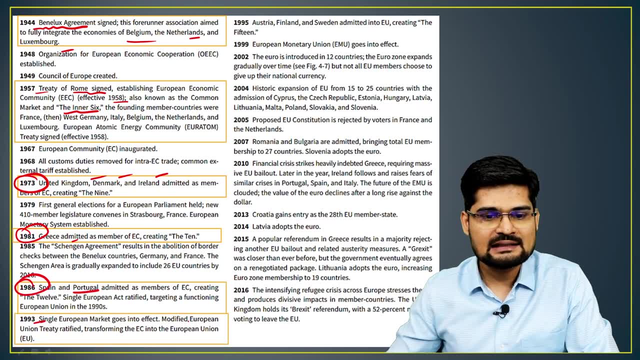 then further, if you observe: united kingdom, denmark and ireland joined in 1973, then further you have greece in 81, then further you have spain and portugal in 86, then you have 1993, the ratification, modern european union treaty, and then what you observe is the monetary union, that is. 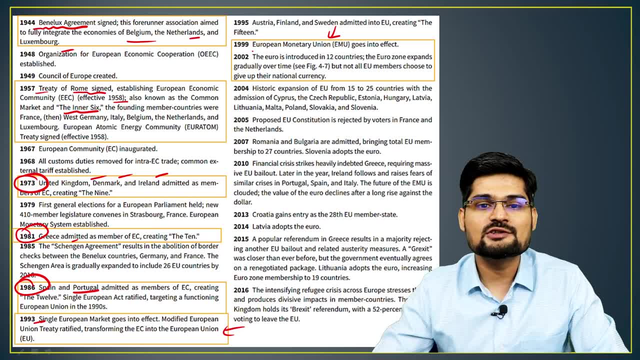 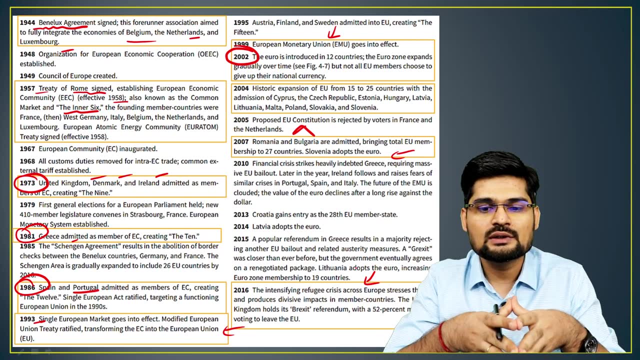 money comes into the effect- emu- and then euro is introduced in 2002- right, and i'm sure you know about these things in history as well. and then you will observe further that romania, bulgaria and other were adopted in 2007 and then further by 2016: the intensification of european union. 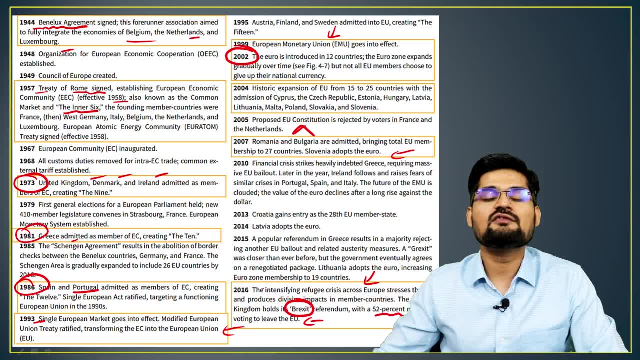 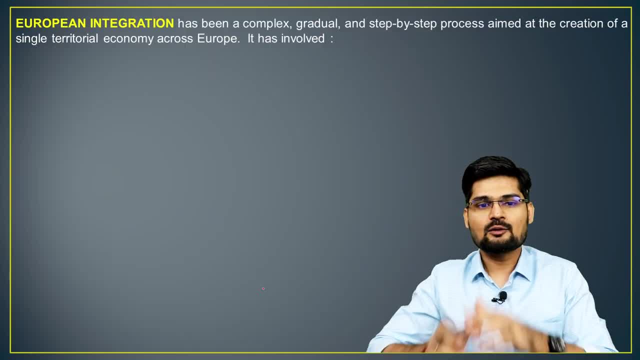 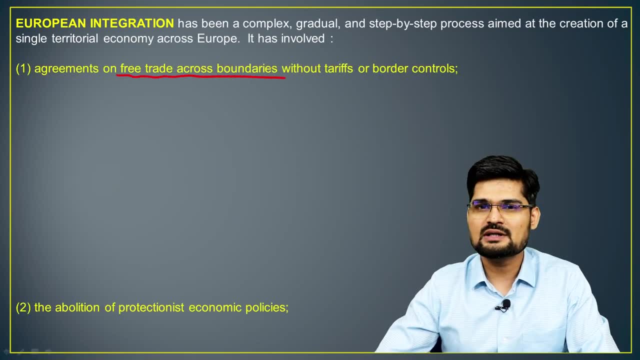 52 percent of majority of united kingdom voted for brexit right. so these are certain things in terms of the political geography of europe as well. if you observe, now european integration has the six major steps that you observe. the first step was agreements on free trade across the boundaries. 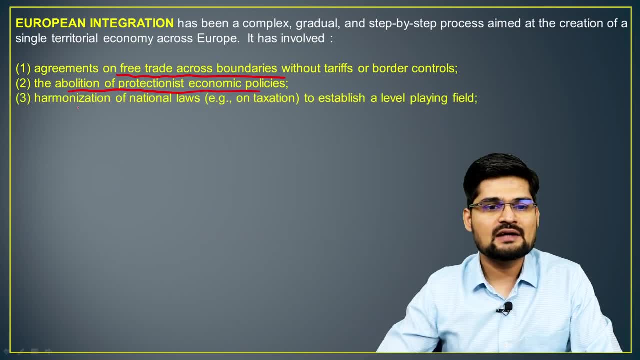 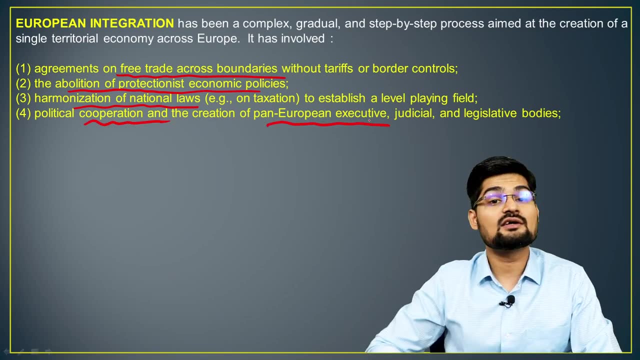 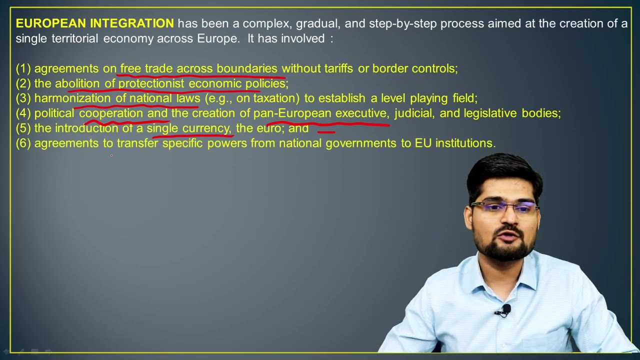 then we have abolition of protectionist economic policies, then we had the harmonization of national laws on taxation. right then we had the political cooperation and creation of pan-european executive, judicial and legislative bodies, and then it was introduction of single currency, the euro, and the sixth and the last step was agreement to transfer. 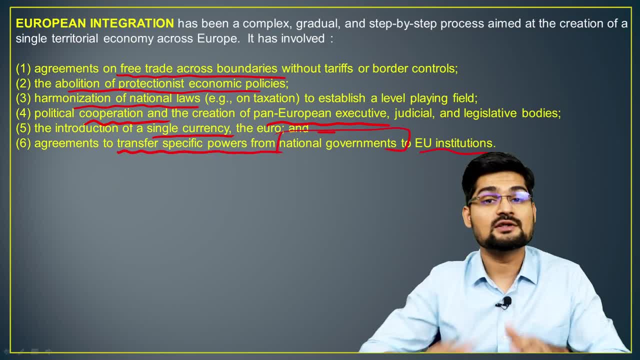 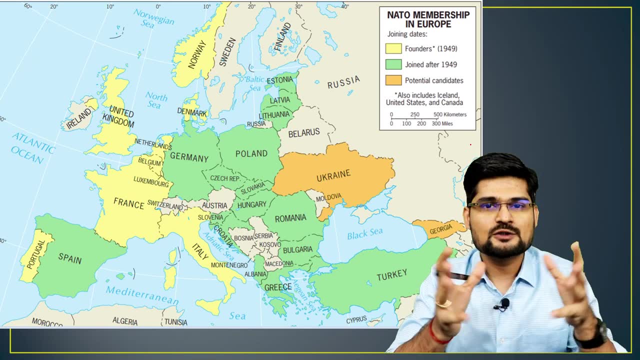 specific powers from national governments to european union institutions. so this is how the integration happened, in these six steps and then further. the nato membership is something that we are also looking into because especially the russia and ukraine war, and who is part of nato? 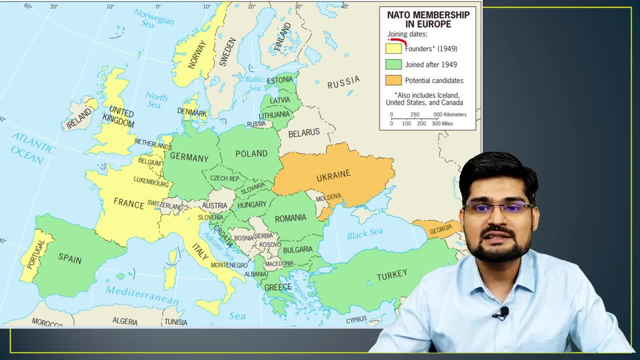 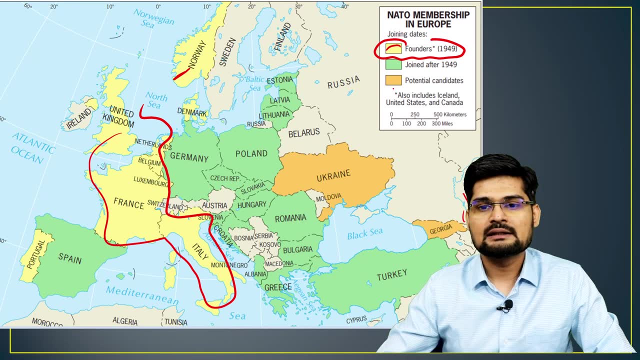 and who is not where the support comes from. so, if you observe, these are the founders in 1949 who were the members of nato earlier, these particular countries out here. then green colors joined after 1949 and right after that the green colors joined after 1949 and right after that the green colors joined after 1949 and right. 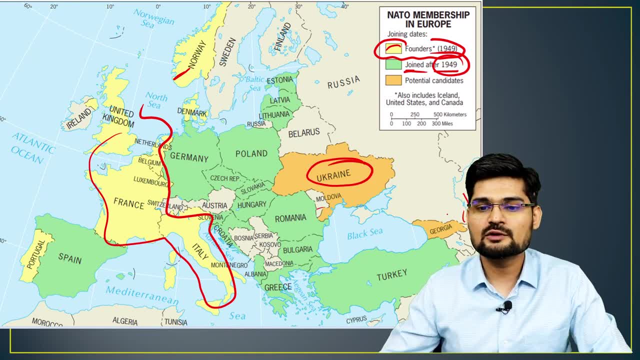 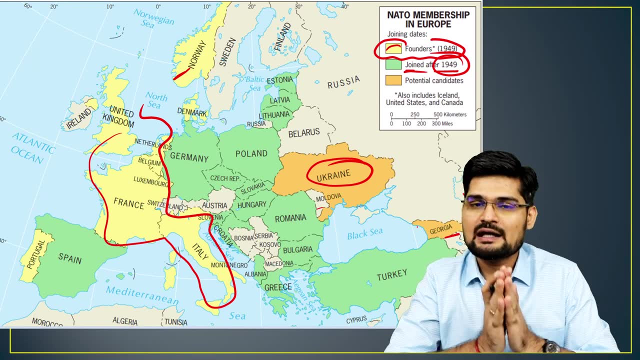 now the talks are that ukraine is going to join, moldova is going to join, georgia is going to join. so these are the countries under which the talks are that they could join nato countries and, as you know, that the russia- ukrainian crisis is going on right now, so this area is under the 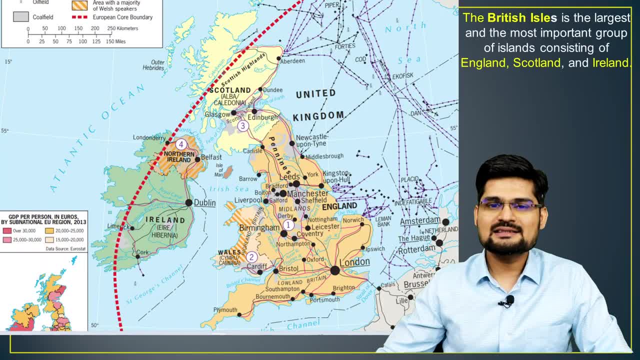 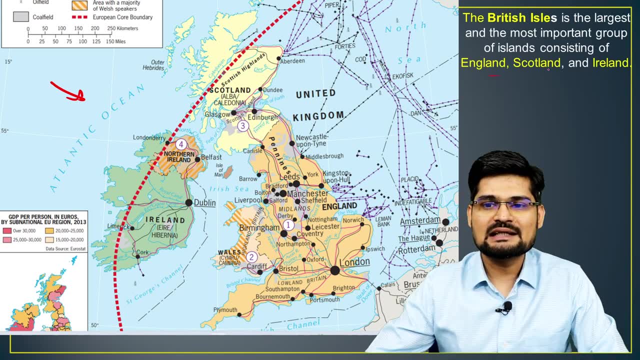 current picture of the world and at last let's understand this particular location which has been the seat of colonialism: the united kingdom. so if you observe united kingdom, the england, scotland, ireland, wales, so scotland is this particular area, edinburgh, glasgow, these areas are important and very famous. the scottish highlands, and then you. 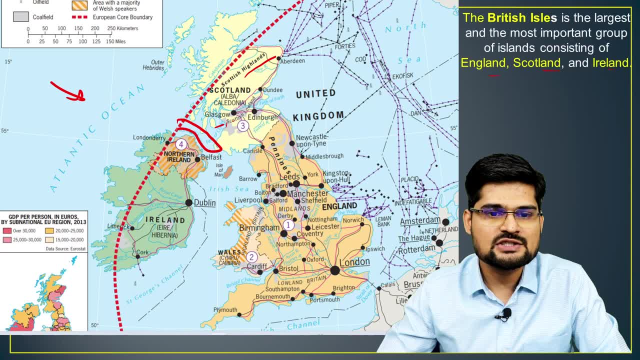 have the other areas nearby it where you see this north channel dividing northern ireland and scotland. here then you have this particular area which is part of the england out here right, and london is part of the southern england. here then you have this particular area called 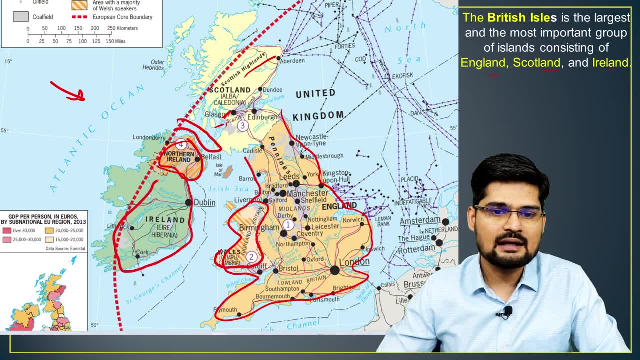 wales. then you have this particular area called ireland. you have irish sea here, the capital is dublin. then particular area, if you observe this part, is ireland. then you have this particular area called ireland. you have irish sea here, the capital is dublin. then particular area, if you observe this part, is: 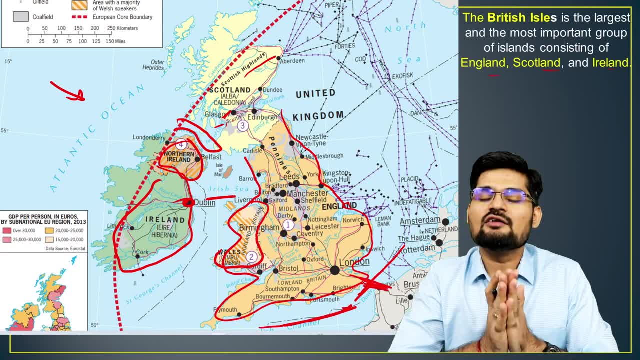 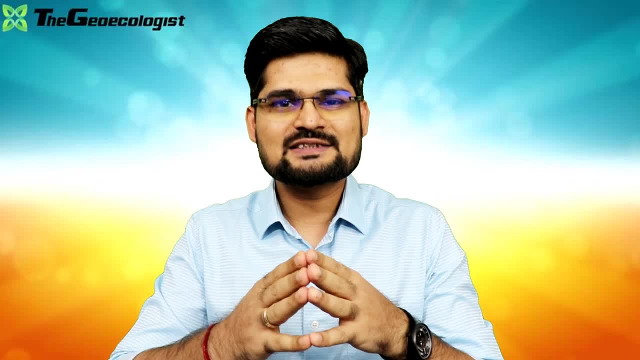 the state of dover english channel, this particular location, very significant area historically, geographically and, right now, geopolitically as well. so now, when we have discussed various aspects of european realm in this session, in the sessions to come we'll be talking more on other aspects of. 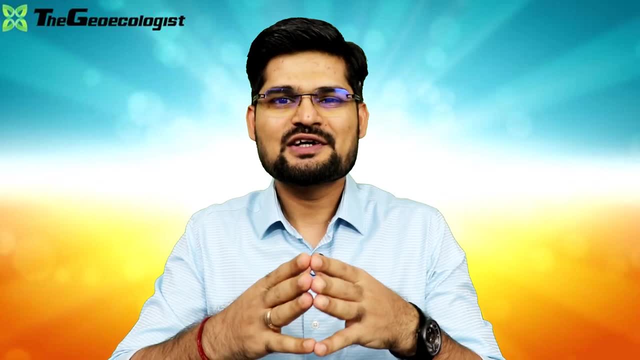 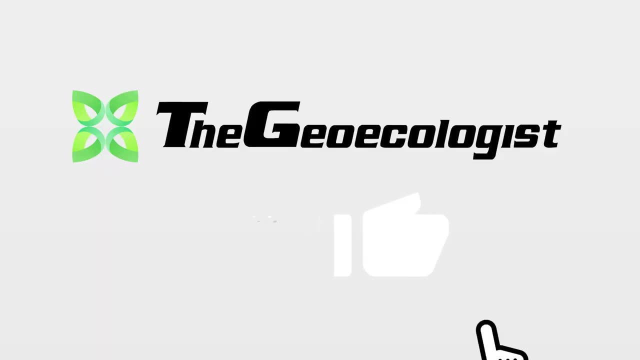 regional geography of the world. so stay tuned, stay safe, keep watching and learning, and don't forget to subscribe to our channel and also, please share the videos with others as well. so thank you so much for watching and i'll see you next time.